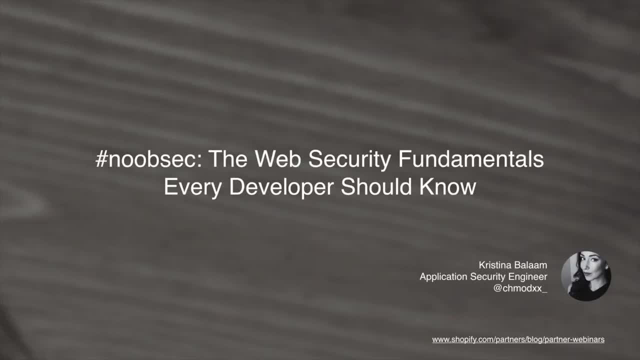 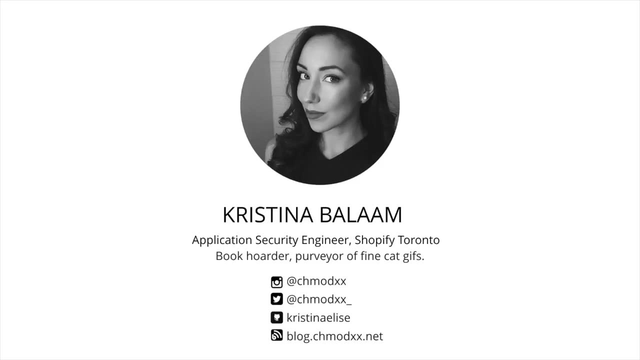 So thank you all so much for coming out to today's partners session. My name is Christina and I'm an application security engineer here at Shopify, And today I'll be talking about web security fundamentals. So, again, as I said, my name is Christina Balem. If you want to find, 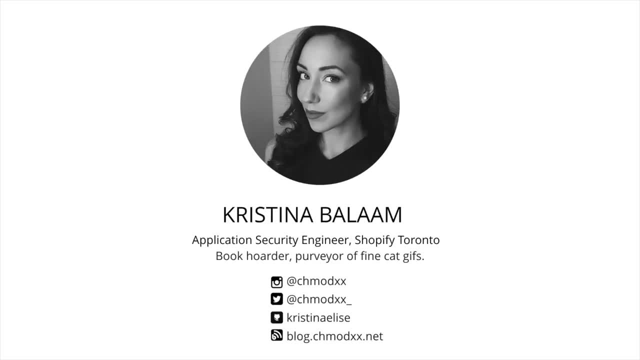 me after the webinar for any questions or follow up, comments or anything like that. I'm on the internet and a whole bunch of different places and you can see them all listed right here on this slide And if you'd like to see the slides themselves, 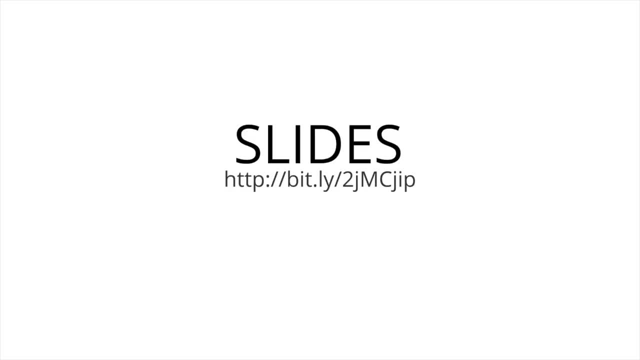 again, they're going to be part of the recorded webinar, but if you'd like to just access them independently, you can reach them at this link. It is. they're basically just uploaded to GitHub's slide sharing application and there's. everything you need is right on there. 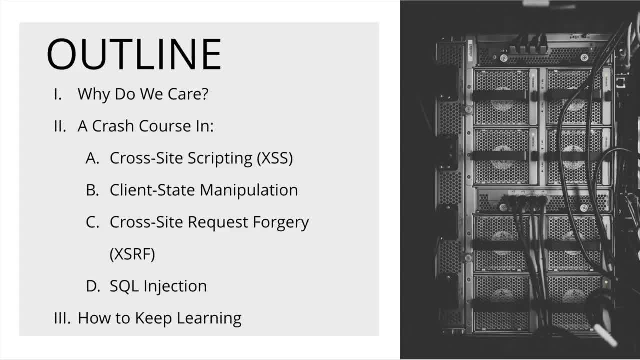 Great. So we're just going to kind of go through a bit of an outline on what this webinar is going to cover, And I really want to emphasize: this is very much a crash course in web security fundamentals. There is so much to learn and understand, but it's also very much a crash course. 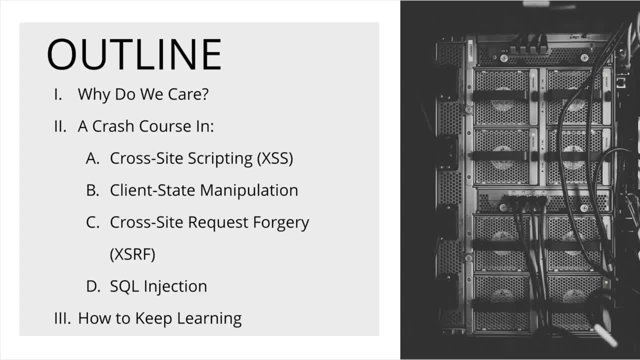 in some of the basic vulnerabilities we see a lot of and how to prevent them. So the first thing we're going to talk about is: why should we care? Why should we care about making sure that our application is totally secure, or at least as secure as we can make it, Especially for those? 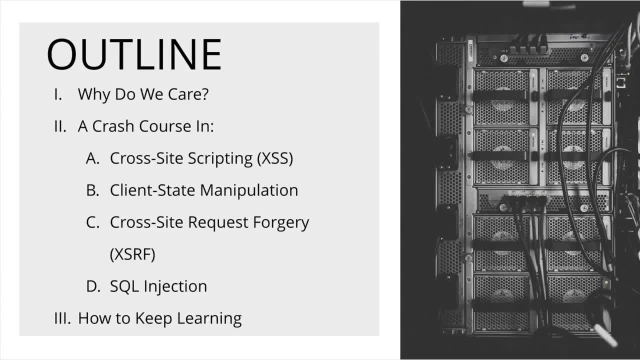 of us who may come from a background of working for smaller companies or agencies. why do we care if someone could potentially hack our web application? if it's a brochure site and we're not actually collecting user data, Why do we need to care about this stuff? Then we're going to jump into. 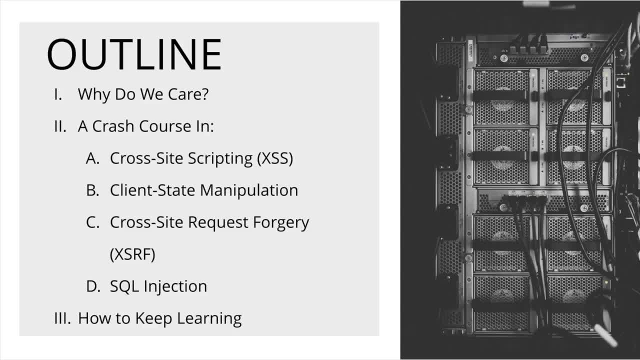 just an overview of four main types of attack vectors in the web sphere. So the first thing we're going to talk about is cross-site scripting, And then we're going to chat about client state manipulation, cross-site request forgery and SQL injection, And for each of these we're going to 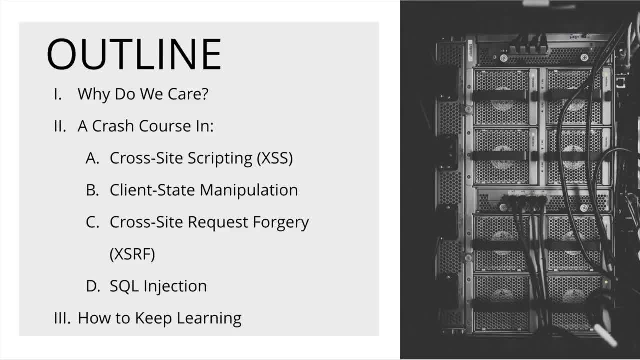 talk about the different types of attack factors that we're going to talk about in this webinar. We're going to talk about what these attacks actually involve and different ways they can be performed. We're going to see a demo of actually performing one of these attacks in a very safe 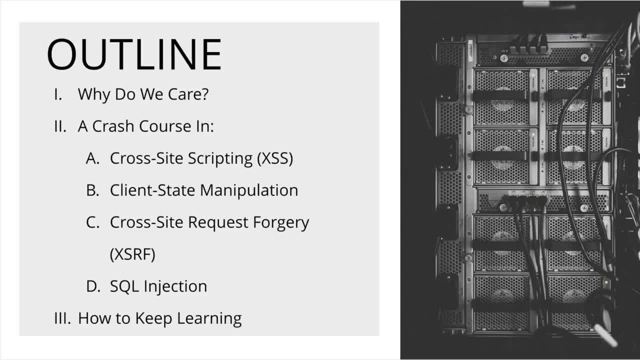 environment on a vulnerable web app, And then we're going to chat about how to prevent them. We're also going to see real-life examples of these happening out in the wild, And they all are accompanied by reports that you can read more about in your time after the webinar. 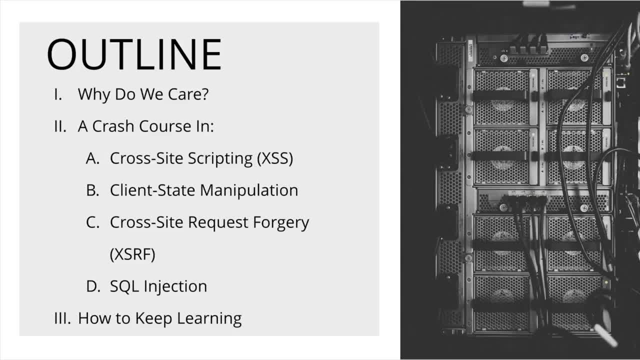 And then, finally, we're going to talk briefly about how to keep learning about these attacks and how to prevent them, And then we're going to talk briefly about how to keep learning. Now, as I've said a bunch of times, this is a very important topic that. 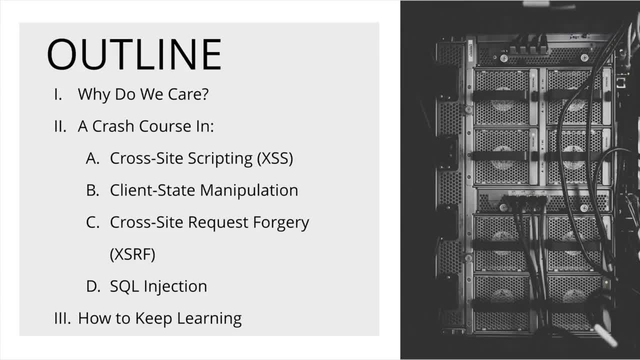 requires kind of a lot of practice, actually, And the more time you spend improving your knowledge of web security and learning from others' mistakes- and learning from your own mistakes you know- the better you can get. So I've listed some resources, some really great books. 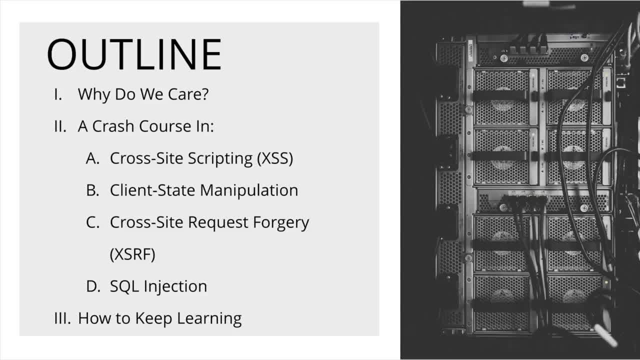 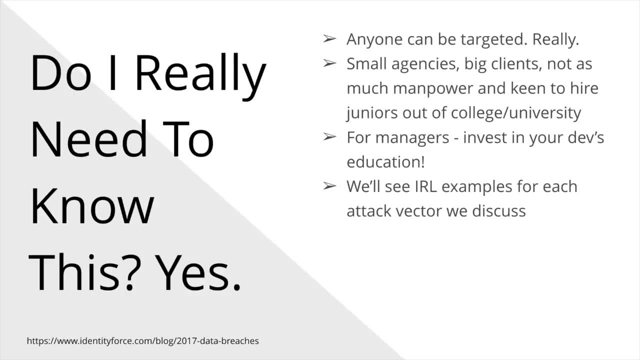 some great courses And we're going to go through those and see how you can basically keep improving after you've learned the basics today, Short answer: yes, You know. security breaches don't just happen to banks and large corporations, And I've heard so many developers say that they don't. 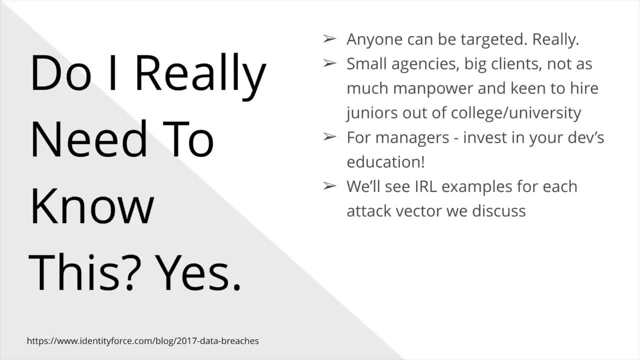 need to worry about some security issue because they're not a target, And at one point in my life I used to think about this as well. But the truth is you don't ever really know whether you're a target, even if your site isn't accepting usernames or passwords And you know it's just a brochure site Data in general. 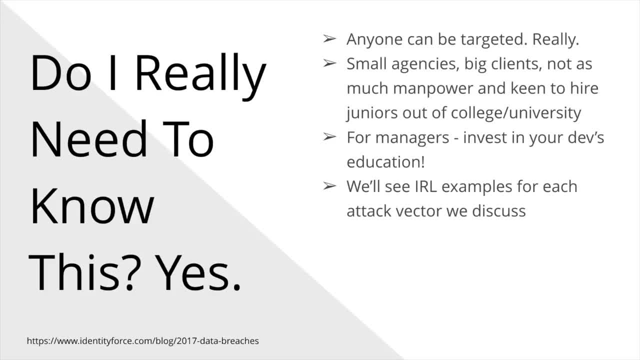 is still a huge asset to hackers. nowadays, Small agencies also, in particular, tend to take a lot of junior developers right out of college or university or boot camp programs, And I know from experience that a lot of those programs don't necessarily focus on security. 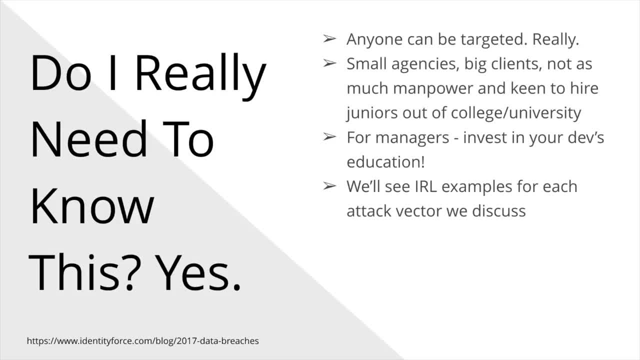 education. In my computer science degree we had a very hands-on program which was great. We wrote a lot of code But really our discussion of web and software security kind of boiled down to theoretical encryption algorithms And that just wasn't really enough to go out into the workplace and 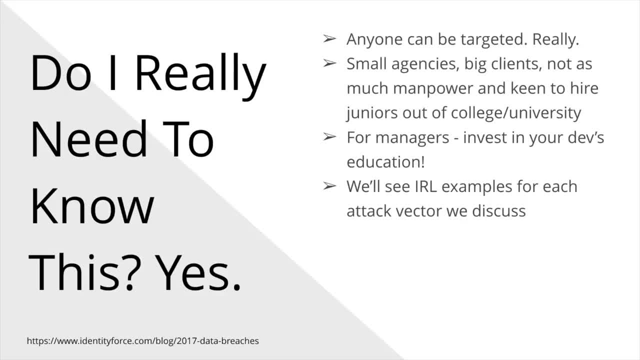 know that the code you're writing is super secure. So, for those of you who are listening in, who may not be developers but may be managers, and you know, even for those of you listening in who are developers and you know might take on a lead or like a VP of engineering role, really invest in. 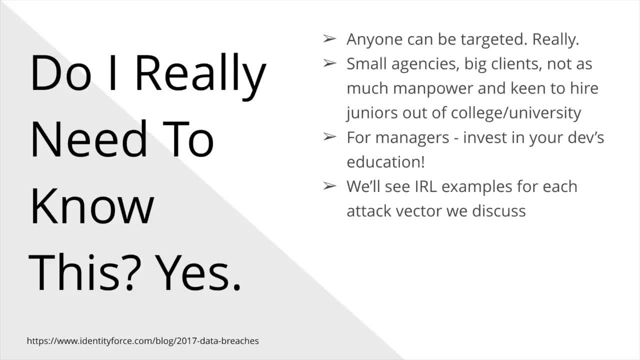 your developer's education. It doesn't mean that you know they need to go back to school and do like a full-blown master's degree in cybersecurity, But there are some really wonderful books. There are some great, you know, relatively inexpensive courses on the internet. There are also some great. 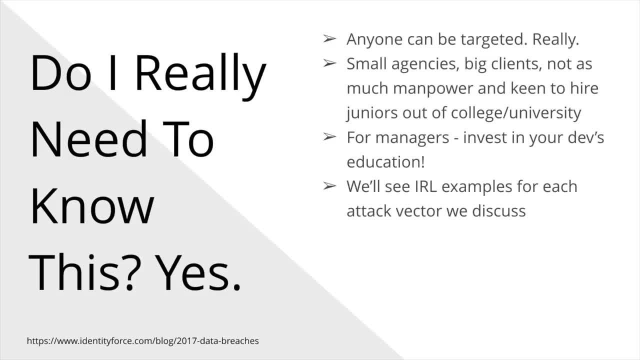 free courses. Coursera has some that are offered by universities or other post-secondary education institutions, And they can be a great resource for developers to really just brush up on the knowledge that they should have learned in school and, you know, maybe didn't. What's really interesting is 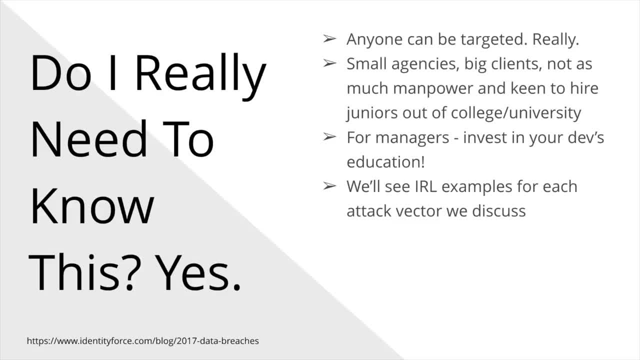 that IBM recently conducted a research study in the United States on cyber security, And it was a really interesting report that was published in 2018. that sort of projected a study outlining the odds and costs of data breaches to organizations of all sizes, And this was done in 2017.. So it's 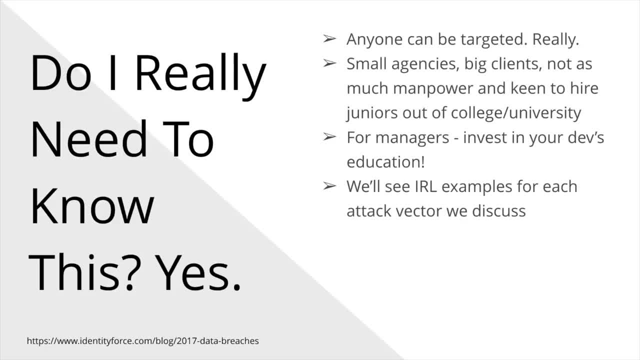 it's current for this year. What's really interesting about this is this report showed that as we progress, as you know, as a society really connected on the internet, the cost to organizations is actually decreasing, So the cost organizations have to pay when they do experience. 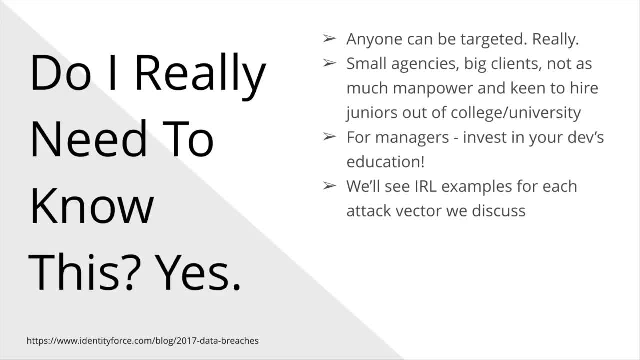 a data breach is decreasing, And they believe this is likely because more organizations are taking preventative measures, And so it's all very clear in the report And that's something that we're measures and employing incident response teams that can contain attacks more easily. 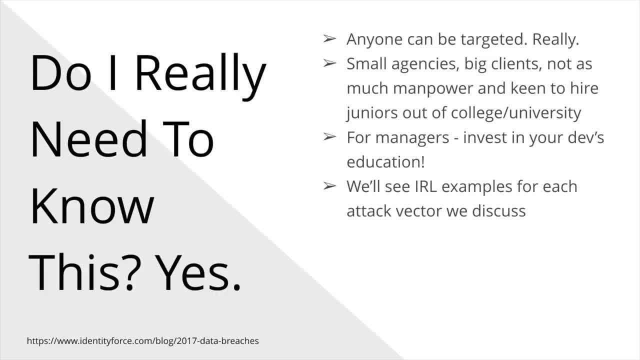 But what's also really interesting and kind of scary is that the average size of data being affected is increasing. The study also outlined that the odds of an organization experiencing a data breach is just one in four, And these aren't, you know, Fortune 500 or publicly traded. 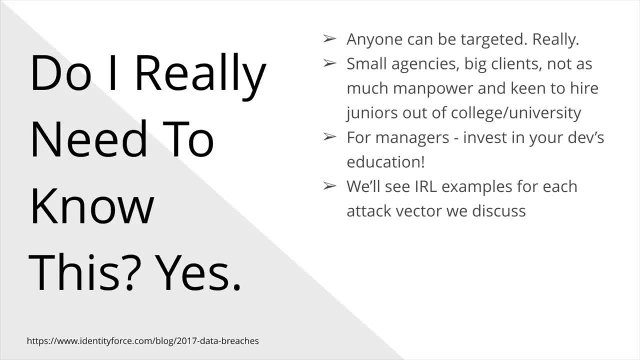 tech organizations that have this potential for data breach. This is really just any tech organization or a company that exists on the web, And I think it's really important for us to discuss security, because security really builds trust with your customers. For us at Shopify, 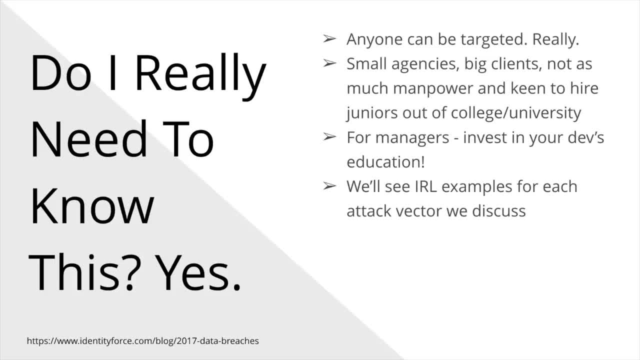 you know, our merchants know that they're on a secure platform And by ensuring that the platform we're providing is secure, we build trust with those people And, in the same way, third-party app developers, you know, provide trust by making sure that they're. 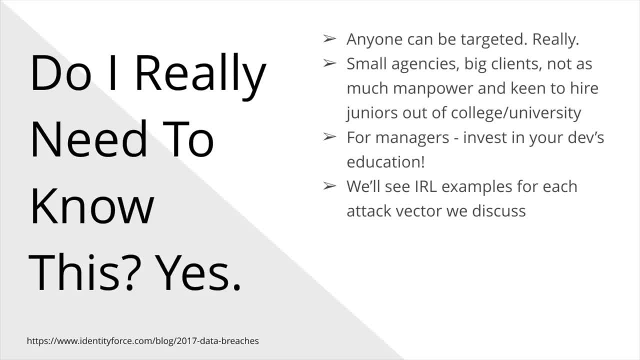 application-friendly, And so you know, I think it's really important for us to discuss security are secure and that the data that merchants may give you access to won't be used in any sort of malicious way and won't be available on the internet somewhere And hackers can't come in. 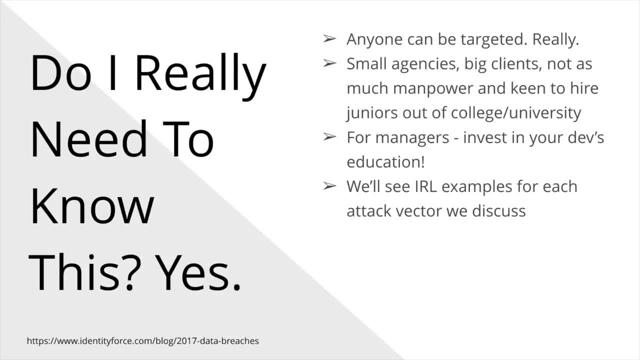 and essentially take advantage of that data. As we've talked about a little bit already, in the world of e-commerce, data is really valuable. So you know, it's not just making sure that credit card numbers are protected- That's fairly obvious- But even the data. 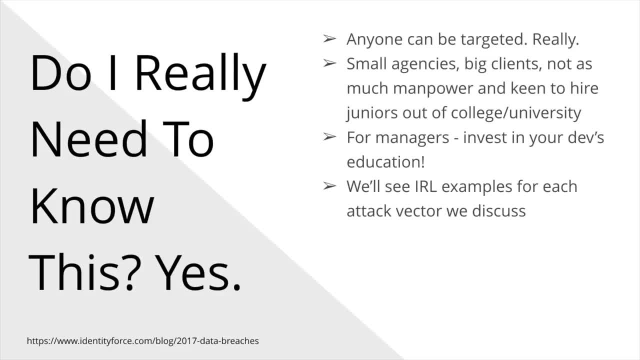 surrounding the number of sales for merchants and the number of customers. that is also very, very valuable information And it can be used in a malicious kind of way by some sort of competing merchant or, you know, angry customer or whatever. So really, security builds trust within an 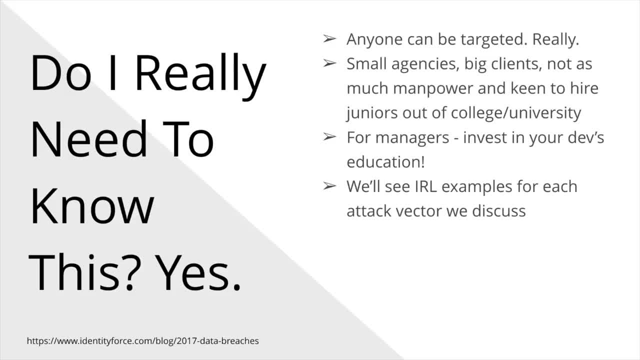 organization and it builds trust between consumers, And it's just really important that we try to make our applications as secure as humanly possible. So now we're going to actually talk about. the first thing we're going to talk about is cross-site scripting. So cross-site scripting. 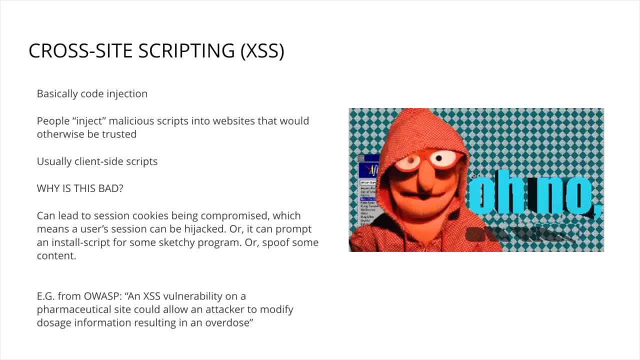 is basically code injection. It's a kind of injection attack where malicious scripts can be triggered client-side by an unsuspecting user. So people may actually trust the website that they're viewing. but if the website is vulnerable to cross-site scripting attacks, then it's possible. 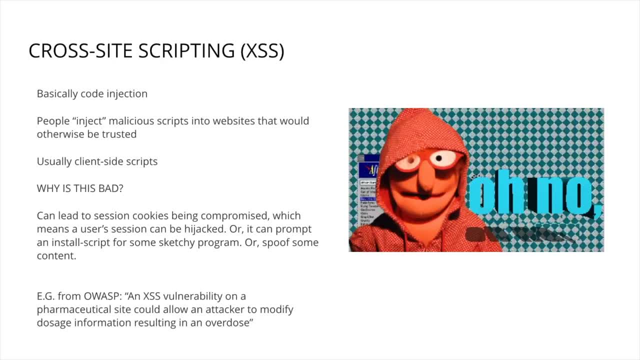 that some other nasty person went in there and threw a little JavaScript script into the site and it could be living somewhere else. So it's a kind of injection attack where malicious scripts can go somewhere in that application to infect or impact other users who unknowingly may reach it. 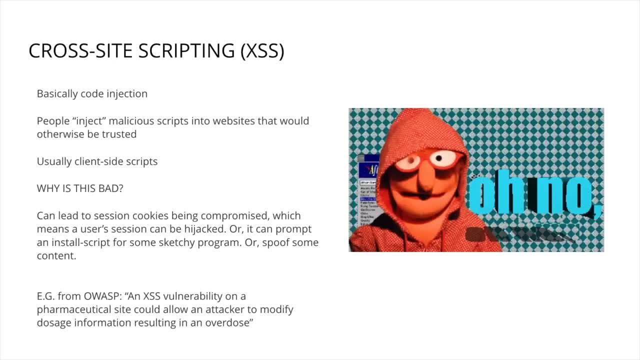 later. Usually, these are client-side scripts, So, as I mentioned, JavaScript is often what's primarily used for cross-site scripting attacks, And this can be bad for a number of reasons. It can be bad because it can allow session cookies to be compromised, which means the user's session. 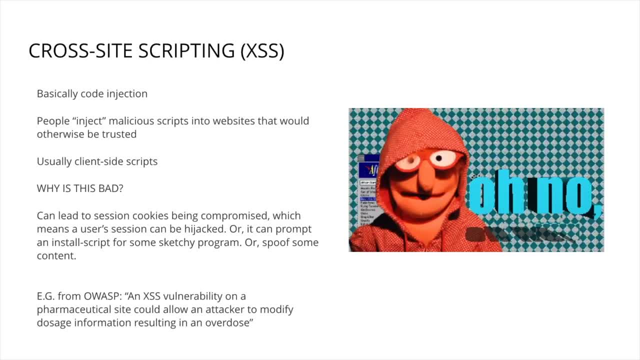 can be hijacked, And I feel like that tends to be a very, very bad thing to do. So if you're using JavaScript, you're going to want to make sure that you're using JavaScript, to be the most obvious example, But it can also prompt an install script for some sort of sketchy program, And we're going 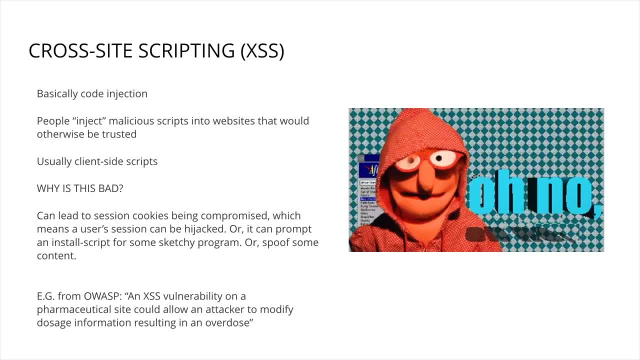 to see an example of how that could happen. Or cross-site scripting can also spoof some content. So one particularly terrifying example for me was from OWASP, which is the Open Web Application Security Project, And we're going to talk about them a little bit in the next slide, because they 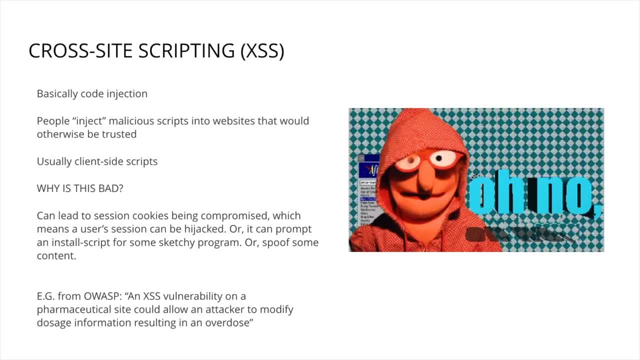 are fantastic, But they've essentially talked about an example of a cross-site scripting vulnerability on what could be a brochure site like a website. So if you're using JavaScript, you're going to want to have a cross-site scripting vulnerability on something like a pharmaceutical site, where you're 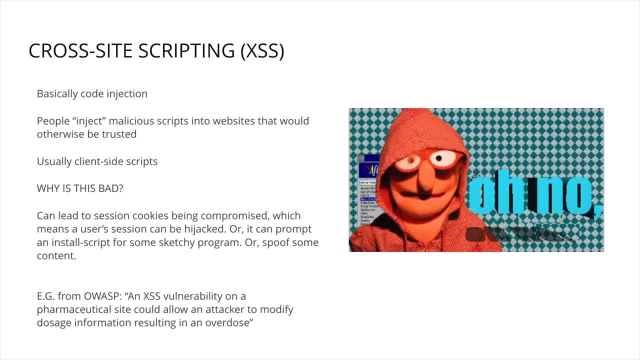 not necessarily taking information from a user, but you're giving the user or consumer a lot of information. So a cross-site scripting vulnerability on something like a pharmaceutical site could actually allow an attacker to modify dosage information, resulting in an overdose, And that. 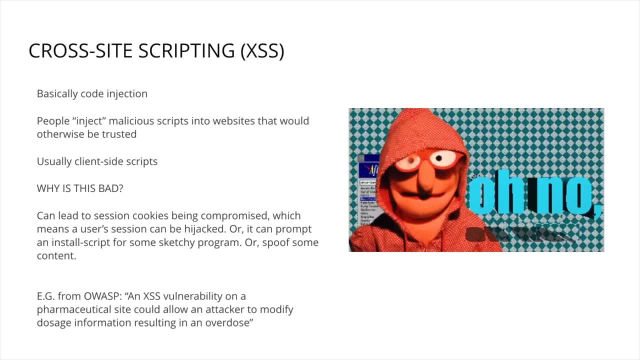 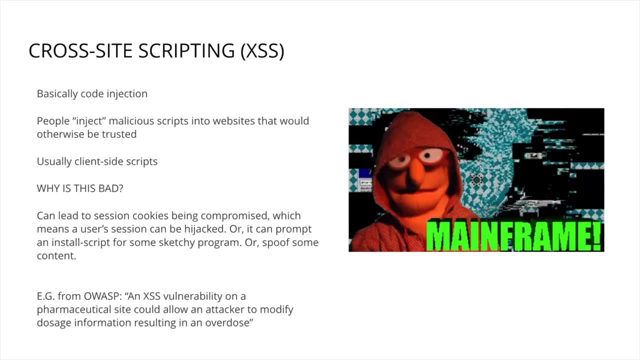 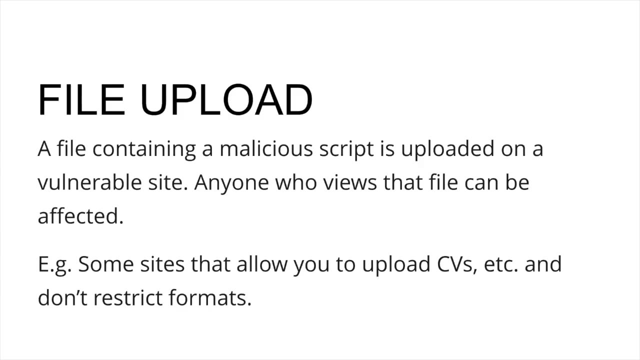 is terrifying, And I feel like it's one of those situations that we don't necessarily think about because there's no actual user data being stored. Oh, there we go. Finally, the GIF is working. So the first type of cross-site scripting vulnerability we're going to talk about is a file upload. 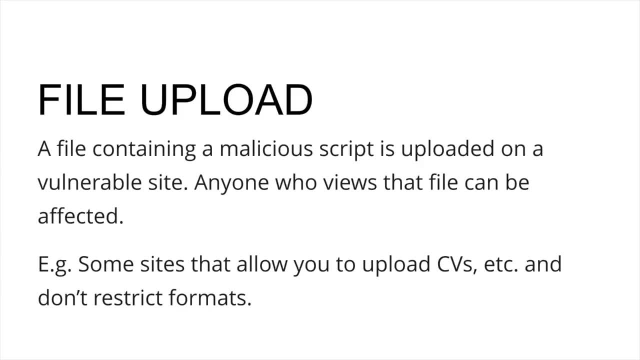 cross-site scripting vulnerability, And this is exactly as it sounds. Essentially, a file containing some sort of malicious script is uploaded on a vulnerable site and anyone who views that file can be affected. So let's say, for example, you have a site like I don't know, LinkedIn, that connects 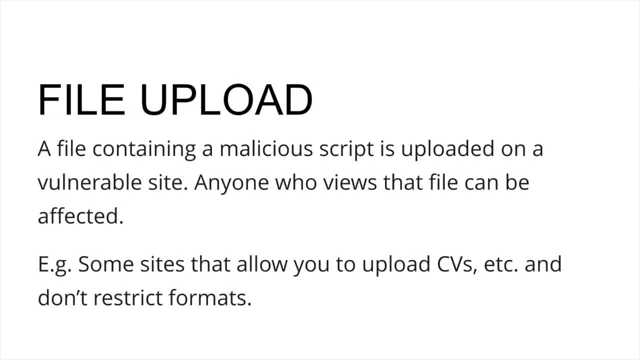 employers and potential hires, And this site doesn't necessarily check what kind of file is uploaded by the user when they upload their resume. The user could potentially upload some sort of malicious script or malware, and then if you have an employer who thinks hey, this person looks like they could be a good fit, let's look at their resume, All of a. 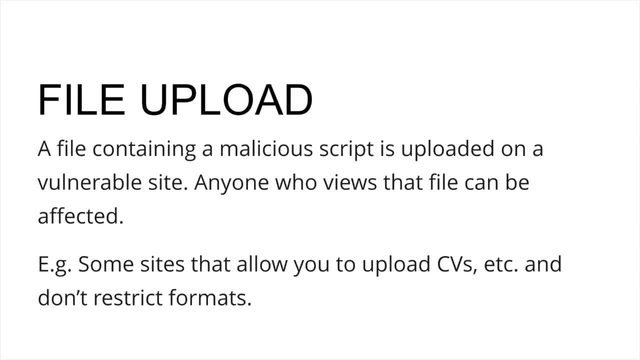 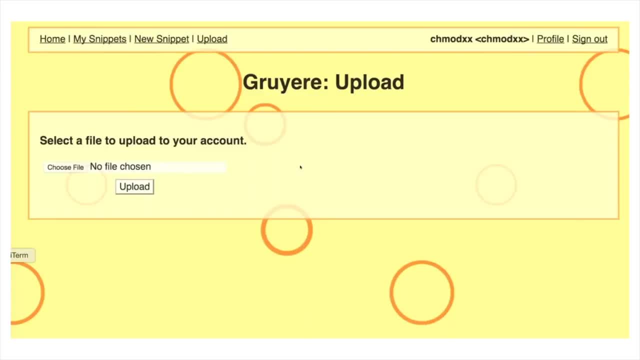 sudden, they've downloaded or accessed that script. So we're going to see a demo example of this right now. There we go. So here I'm creating a dummy HTML file that's going to trigger a script with an alert that 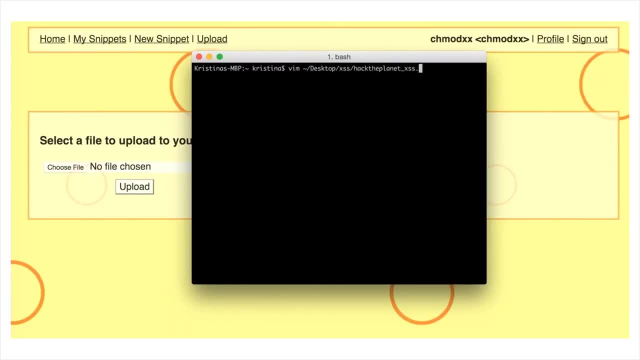 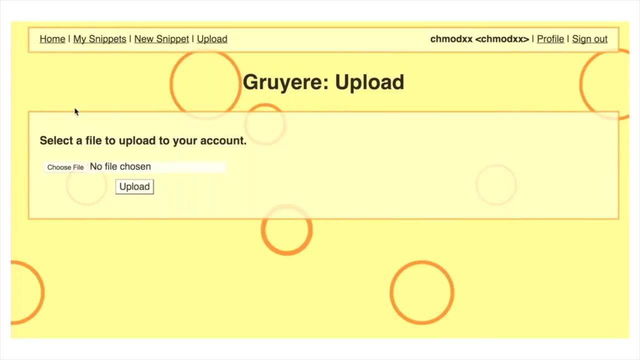 will just show the current user's cookie. We're not really doing anything malicious, demonstrating that you can actually trigger some JavaScript that really is not supposed to be there, And this will demonstrate that there's a cross-site scripting vulnerability. So we've got our basic little HTML file and now I'm going. 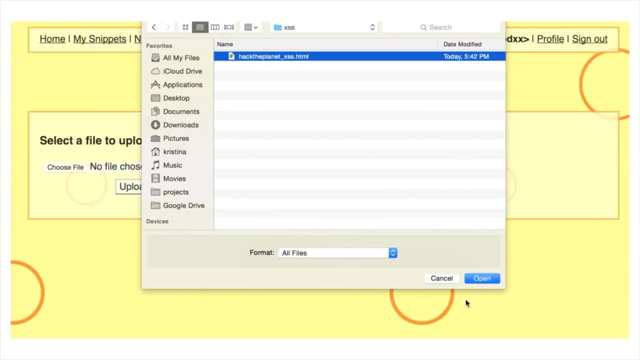 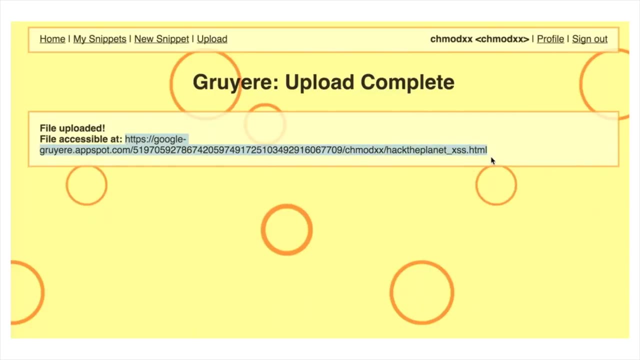 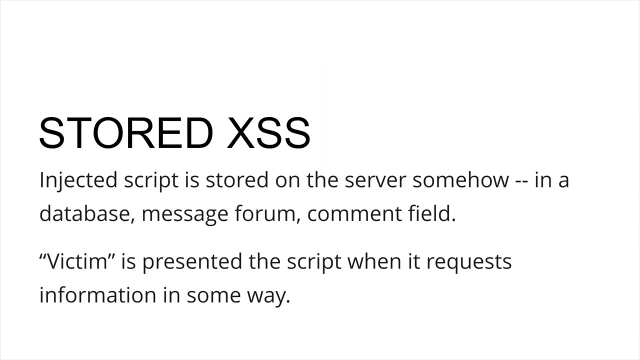 to upload it And there's no problem, because they're not checking that it is actually some sort of appropriate file. So now, if I go to that particular file, there is my cookie And that is demonstrating a cross-site scripting vulnerability. So now we're going to move on to stored cross-site. 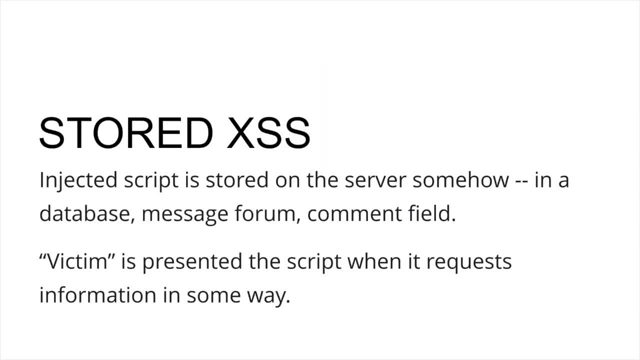 scripting, And this is when the attack is stored somewhere in the application and the victim triggers it by accessing a page that renders whatever malicious script has been uploaded, So it lives on the server somehow in a database or a message forum or a comment field or any any one of those you know forms that may. 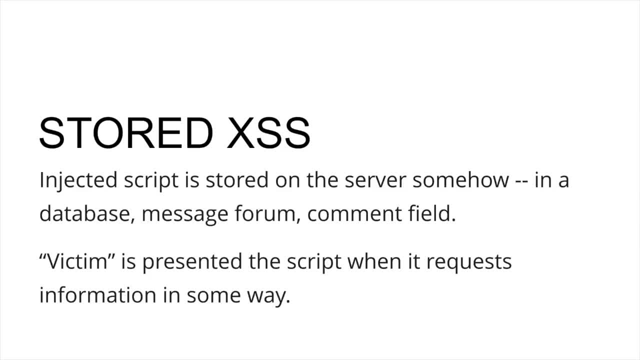 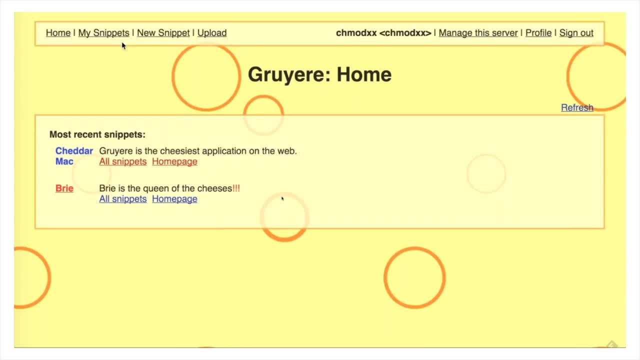 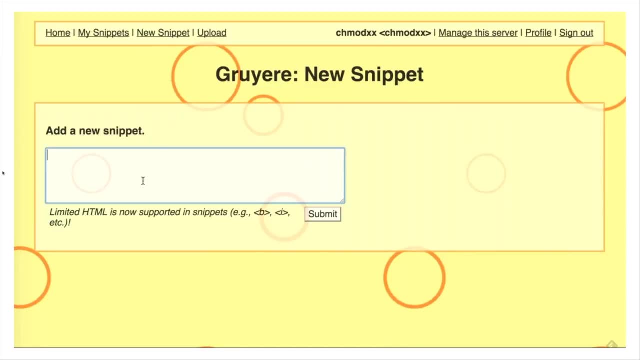 be stored in a server somewhere And then the victim is presented the script and bad things happen. So we're going to see another demo outlining this And again we're going to see the alert script with the session cookie. So I'm storing this potentially malicious. 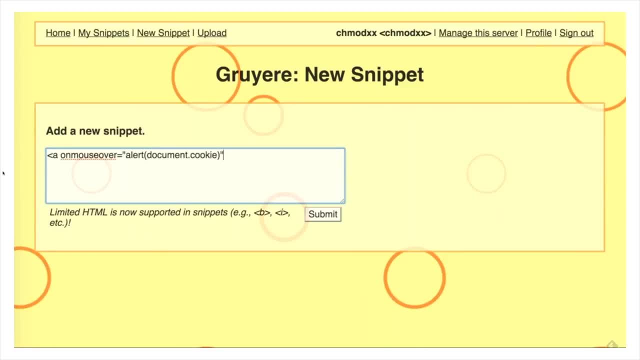 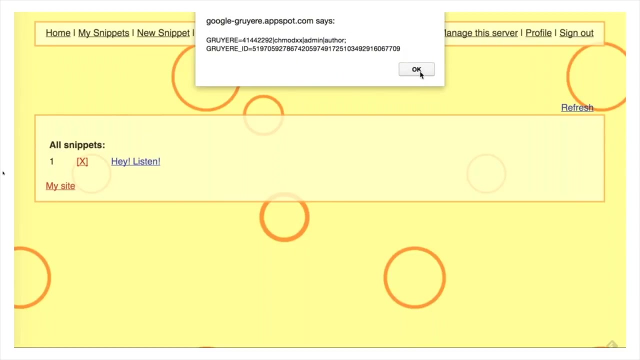 script as a little snippet, And in this context snippet is sort of like a github gist And this gets stored to the the web app database. The form allows us to write this script. It doesn't strip out the actual functionality. So when I mouse over, there is the cookie again, And 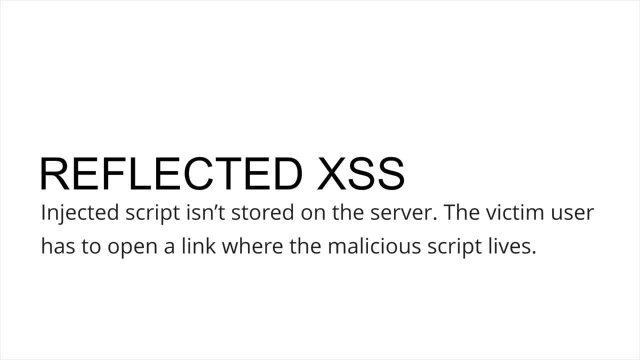 finally reflected cross-site scripting attacks. So this is when the injected script isn't actually stored on the server. It's where the victims lured into making a request to the vulnerable application and the script is injected by, say, like a parameter of that request and then returned immediately as part of. 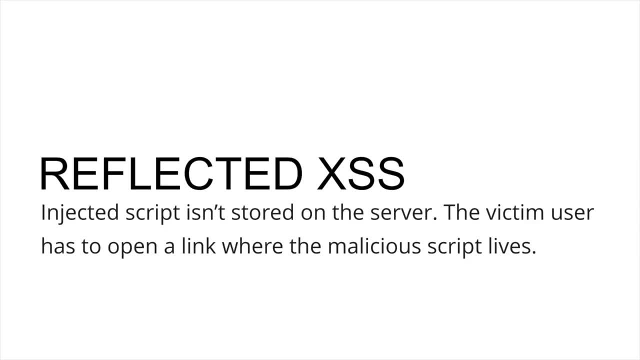 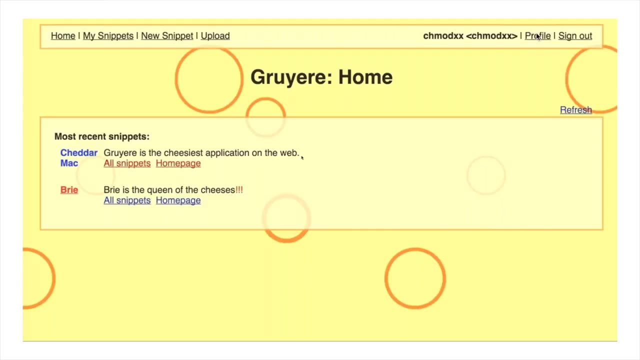 the response So stored. cross-site scripting involves scripts that are delivered sometime later after the system was infected, And reflected cross-site scripting attacks happen right away for the user. Here we're going to see a simple example of a reflected cross-site scripting vulnerability, And one good example is with profile forms that don't validate. 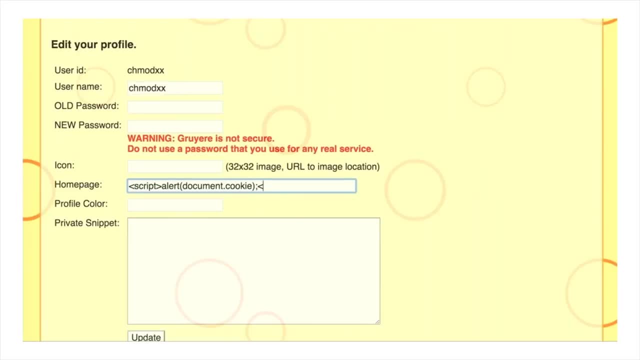 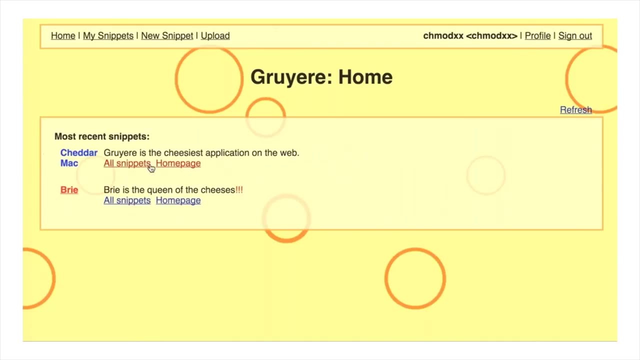 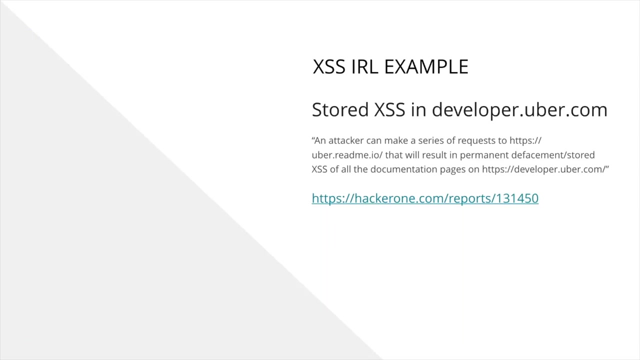 or escape input strings. So here in the homepage URL input field I'm just going to throw in a little content JavaScript alert. So now, if someone goes to look at the profile that I've created and says, hey, let's go see what her site's about, all of a sudden there is their cookie. 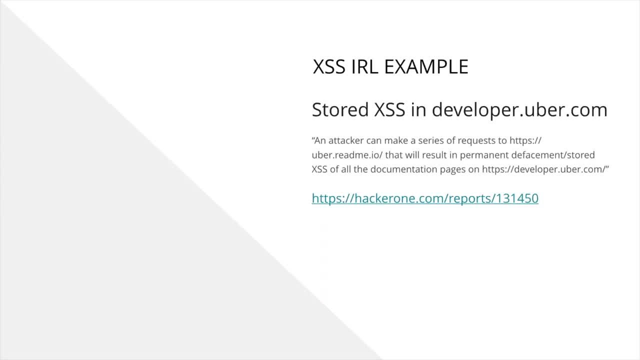 So an example of cross-site scripting in real life is outlined in this HackerOne report. For those of you who haven't heard of HackerOne, it's a bug bounty program and it's the one that we use with Shopify, and essentially what it allows people to do is ethical hackers. 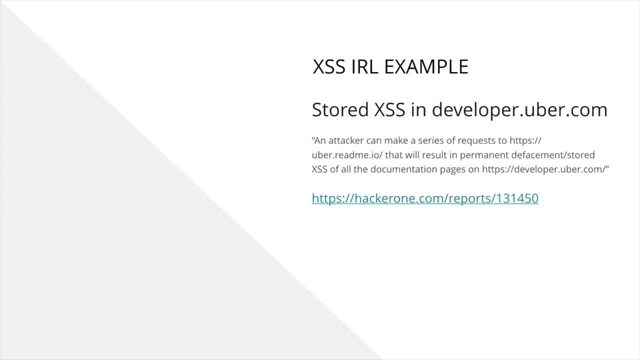 and researchers are able to look at certain applications that have signed up for HackerOne, find vulnerabilities and disclose them in reports that say, hey, we found this vulnerability. we think it does this. here are the steps that I took to recreate it and take a look. 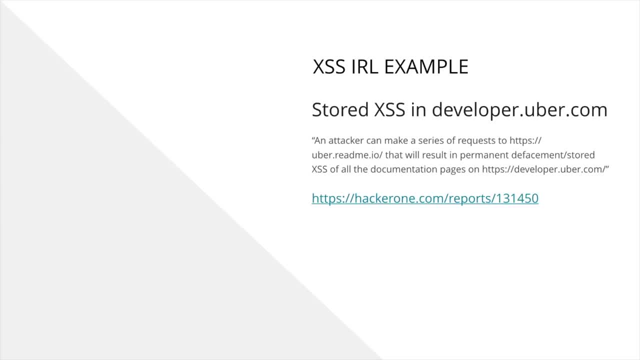 and hopefully I should get some money from it. So this is one example of that kind of report and this was for Uber and this was on Uber's developer site. So Uber had a readme file that it was allowing people to submit suggestions to and what 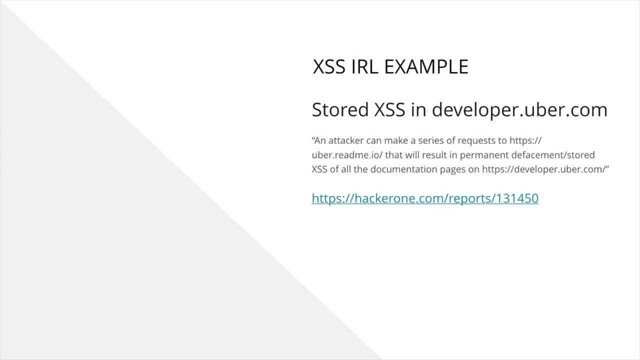 happened is that you can load the readme file, the readme doc, and you get an SID cookie. So when you authenticate your session and you send a request with the appropriate cookie that you've already been assigned, you make a legitimate request. the response you get: 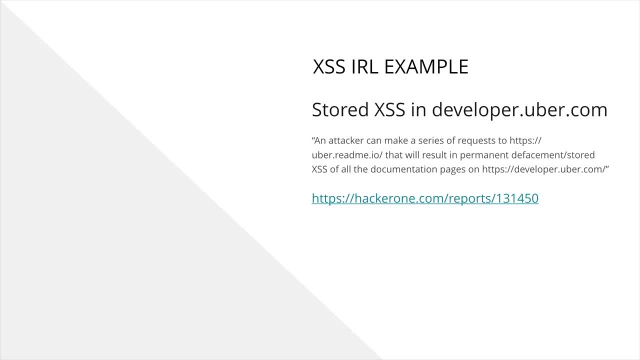 back gives you a new SID cookie, but then you can use this to load an edit page where you can submit suggested edits. Now the problem with this is that any attacker could add some random payload to the form that's being submitted as a suggestion to the Uber docs, and then this is submitted. 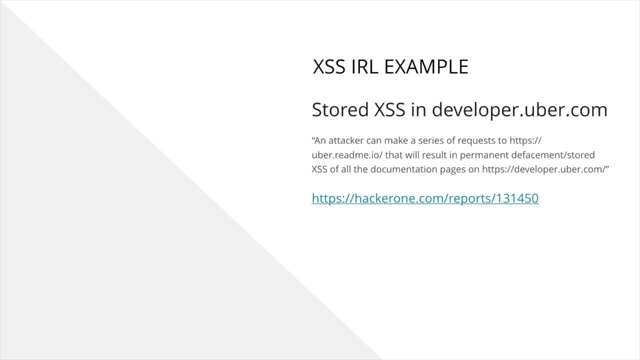 to some kind of administrator or whoever monitors the readme documentation to decide whether the suggestion is actually valid. And why this is scary is that the injected script could actually auto-approve the suggestion, which is then accessible to anybody who goes to the developerubercom. 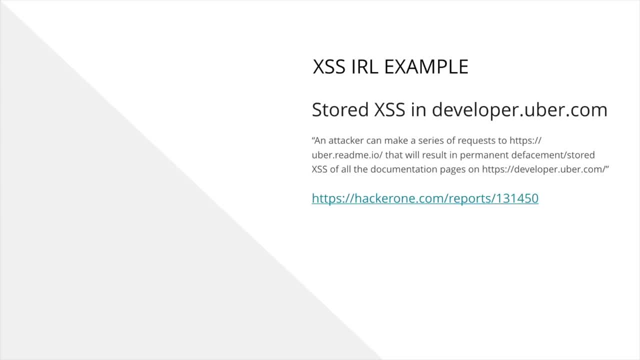 Okay, So this was a big issue. The ethical hacker received $7,500 for disclosing this vulnerability and it's a really good example of a stored cross-site scripting attack in real life and I really suggest you take a look at that report because it's very interesting. 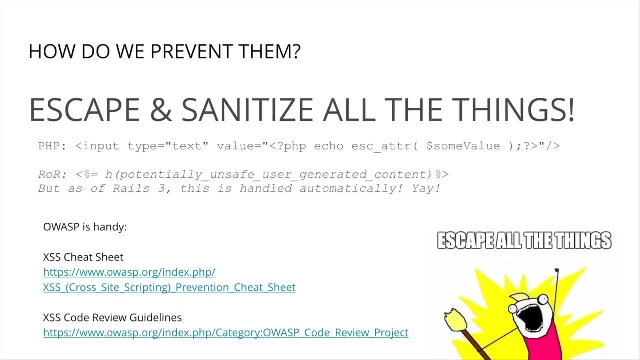 So how do we prevent this? The simple answer is to escape and sanitize all the things. So if you're taking input from a user, you're going to have to do a lot of things. So if you're taking input from a user, make sure that you are sanitizing that input to. 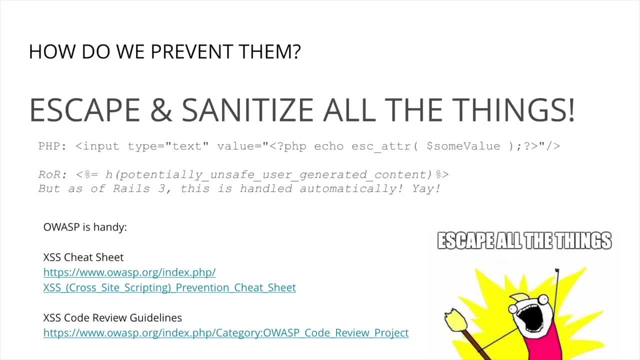 prevent users from submitting, you know, JavaScript little snippets or other kind of malicious content, like we saw with the mouseover that was being submitted with that little snippet in the previous example. In PHP, this looks something like this escape attribute function In Ruby on Rails if you're a Rails developer. what's great is this is actually already handled. 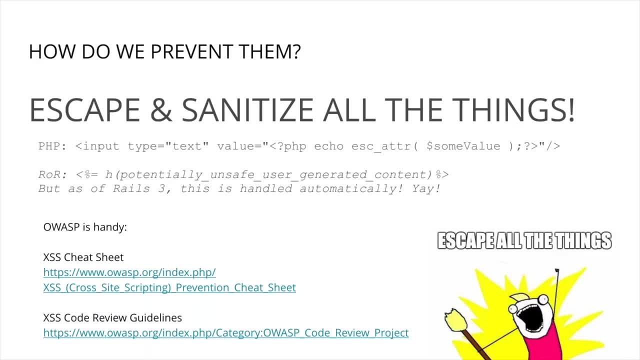 as of Rails 3.0. So you don't have to worry about it. It's handled automatically. For those of you working in different languages or wanting to learn more, I really suggest you check out this cross-site scripting cheat sheet. Again, OWASP, who I mentioned before, the open web application security project. they 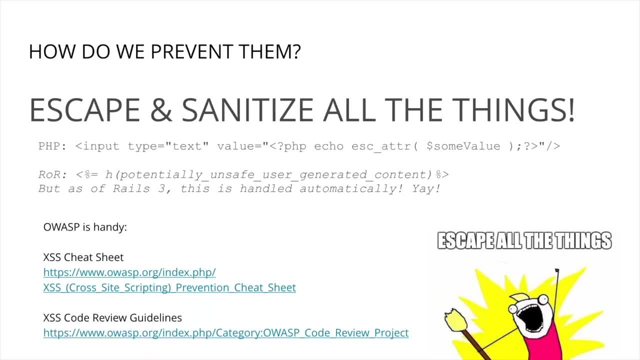 are fantastic. They have incredible resources, And this cheat sheet really gives you pretty much all the information you need to know in order to prevent cross-site scripting attacks on your web application. Another great resource is this code review guideline that they have also made public. 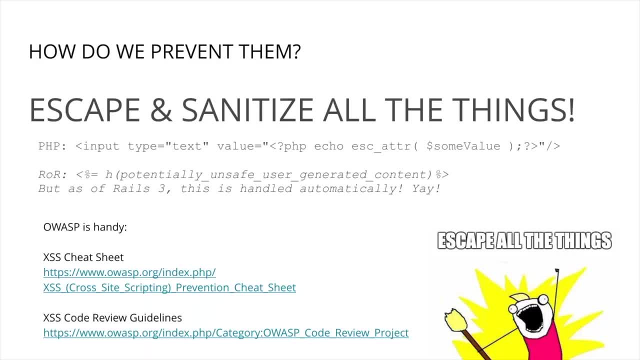 and for those of you who are leading code reviews, this is a great way to kind of go through whatever code is being submitted with your project and make sure that the code being written and developed by your developers actually meets the guidelines that OWASP suggests. 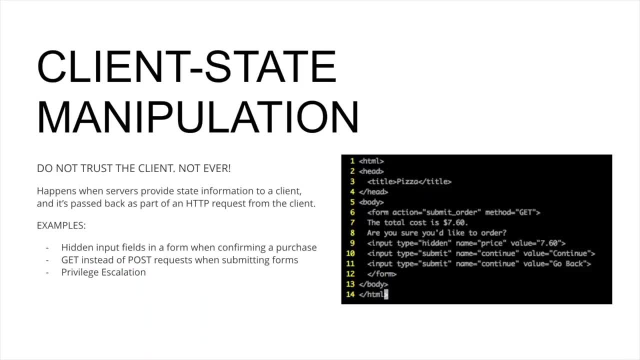 So next we're going to talk about client state manipulation. So this happens when the server provides state information to a client and then it's passed back as part of a request from the client and the client is able to do nasty things with it. 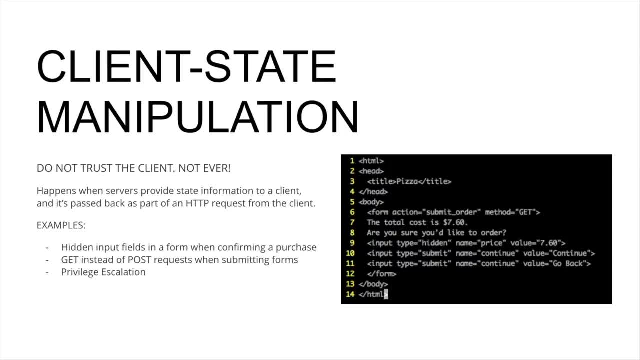 So the lesson from client state manipulation that I'm going to say probably about four times over the course of the next 10 minutes while we discuss these slides, is: do not ever trust the client. Never, ever, ever, ever trust the client, And we're going to see examples of why. 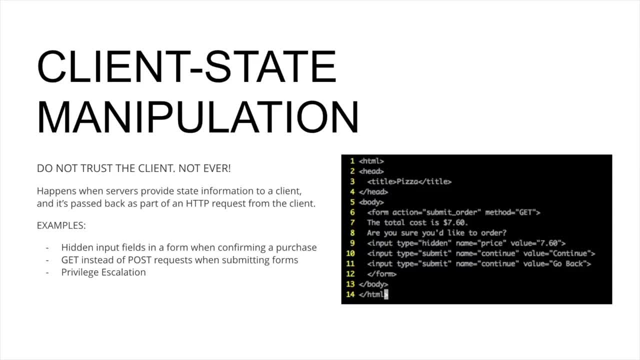 There are some really, really horrible things that can be done with client state manipulation. One very simple example: that likely wouldn't happen nowadays, because I think most people taking credit card information normally use some pre-existing tools- Software- But let's assume that some pizza place like a mom and pop pizza shop down the street built. 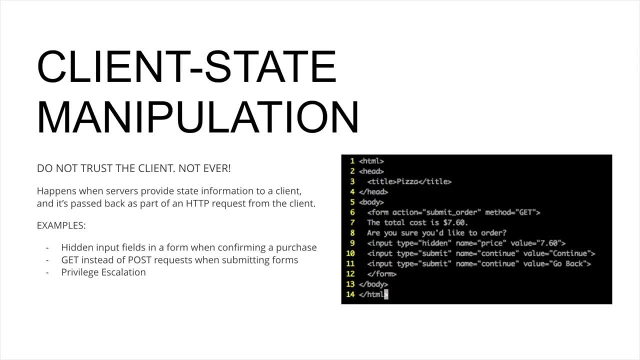 their own website and they're taking pizza orders. Now let's assume that if you look at this little code snippet on the right-hand side here, let's assume that they have a submit order action and they're submitting this all with a get request. but even if it was a post method, it would still be incredibly. 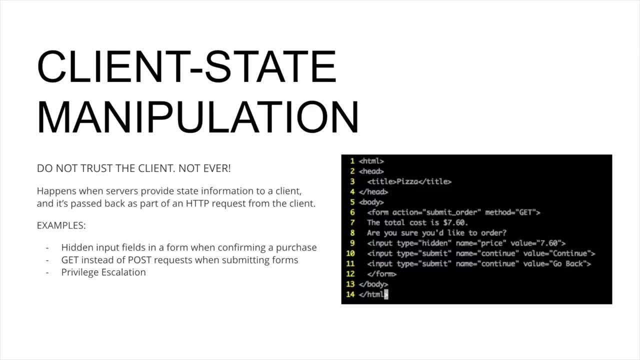 dangerous. So we see that You know Presumably at this point in the application the user has gone through and selected what kind of pizza they'd like and they meet this pizza order form page that says the total cost is $7.60.. 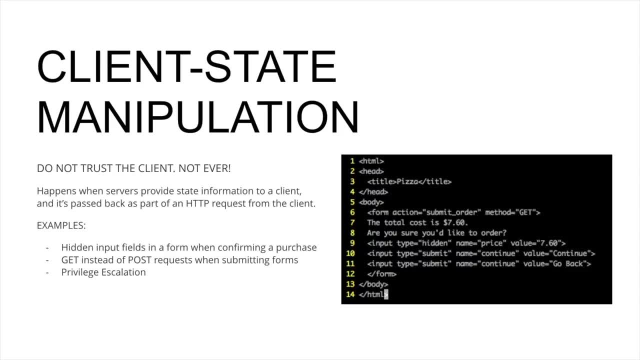 Are you sure you'd like to order. Then the user can either submit and continue to actually place their order, or they can go back and make some changes. Now, if you look at this, you also see that there's a hidden input type that handles the 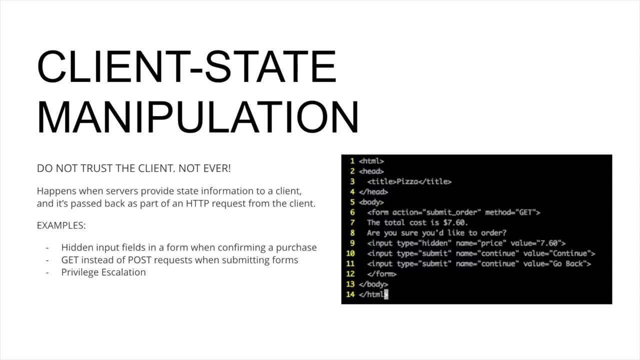 price. Now, the problem with this is that hidden input fields on a fork. I'm going to show you how to do that. So if you have some sort of malicious user who's like, I don't want to pay $7.60 for. 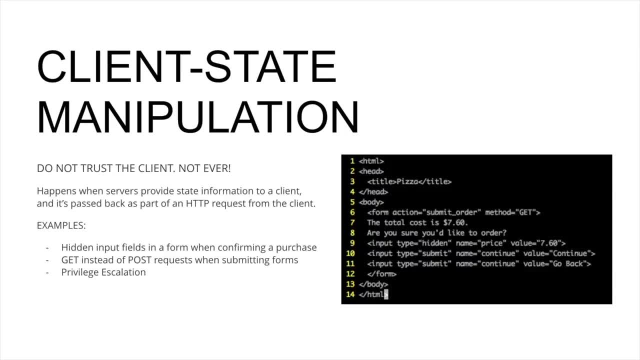 a large pizza, I want to pay $1.20.. They could actually go inspect the document, inspect the page, change out the value to be $1.20, and then continue on with this process as though nothing had actually gone wrong. 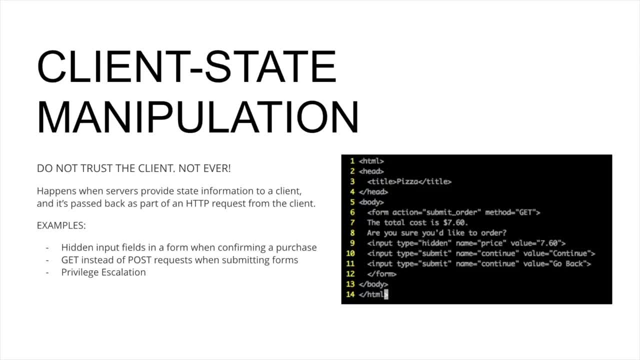 So all of this data would still be submitted to the server and this poor mom and pop pizza shop would be out. you know a whole lot of money if this happened a whole bunch of times. So if you look at this, you can see that there's a lot of data. 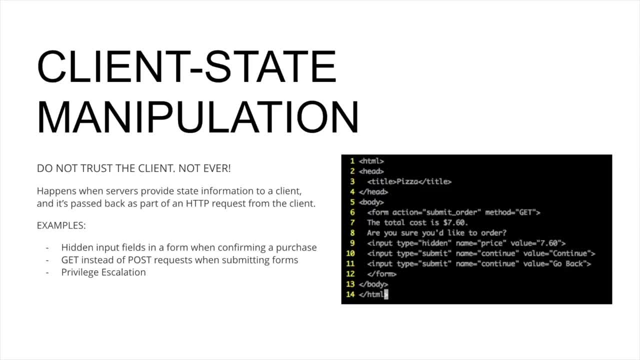 There's a lot of data. There's a lot of data. There's a whole bunch of times. So this is a very simple example. Again, we probably wouldn't see this as much nowadays, because a lot of the time when you're taking credit card payments online, people are using more secured software. 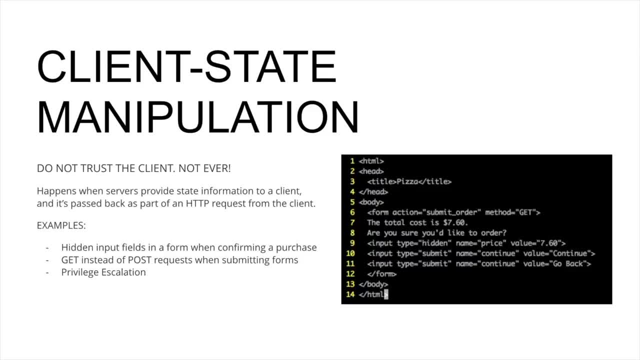 But, in all honesty, I have actually seen this kind of thing in my life. before Shopify, while working at an agency and looking at other existing applications, I've seen people use PayPal buttons And the PayPal buttons were actually Like: the data associated with the PayPal button was being populated from an input field. 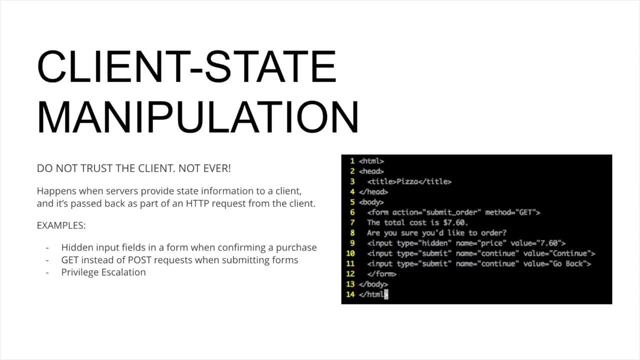 that was hidden but not secured and not validated in any way. So even if you are using something like you think, hey, PayPal's trustworthy, it's still really easy to get around some of those, like you know, quote unquote- security measures. 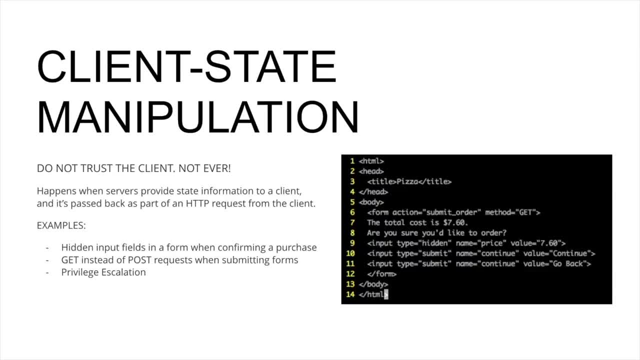 of using a piece of software like PayPal, So that seems like it should be secure. It's really difficult to actually pass any sensitive information to the client without it being manipulated or potentially manipulated in some way. The other issue we're going to talk about that can result from client state manipulation. 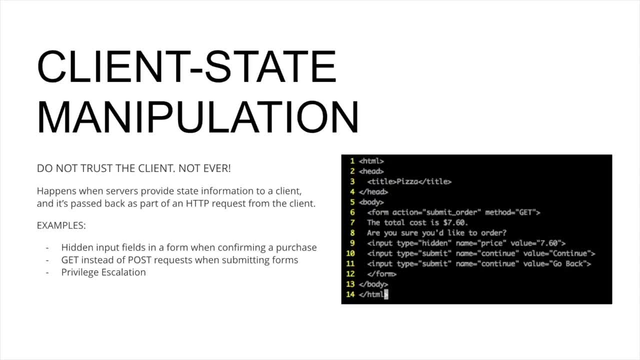 is privilege escalation, And this is a huge issue And we're going to see an example of that coming up. But if the server isn't validating requests, then you can easily modify your existing account information to become an administrator, And that's bad for a whole bunch of reasons. 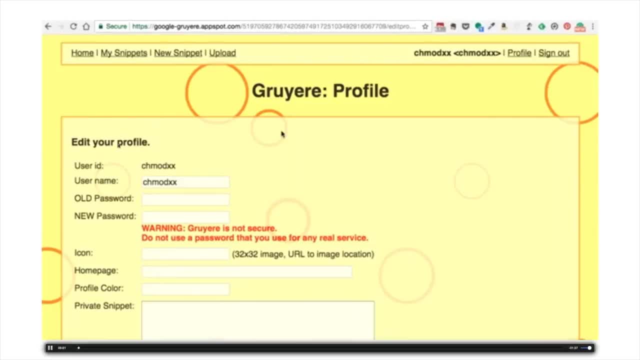 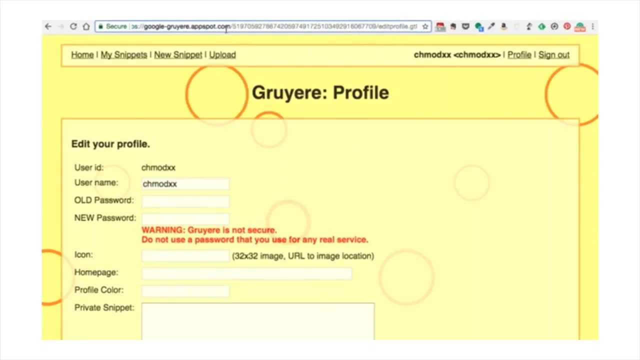 And we're going to see that. We're going to see that right now. So here I've logged in to my little site and I'm just clicking around to see what I can do. OK, so I see that I'm on the Edit Profile page and there's that big log number. 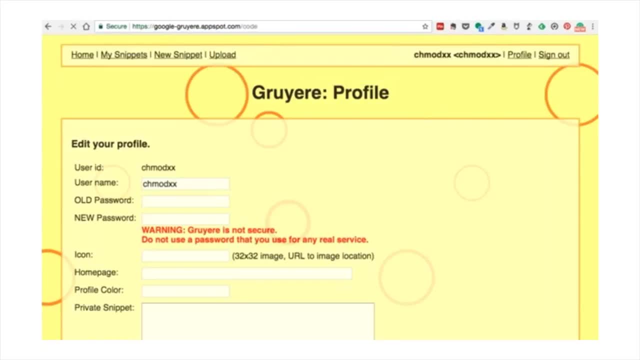 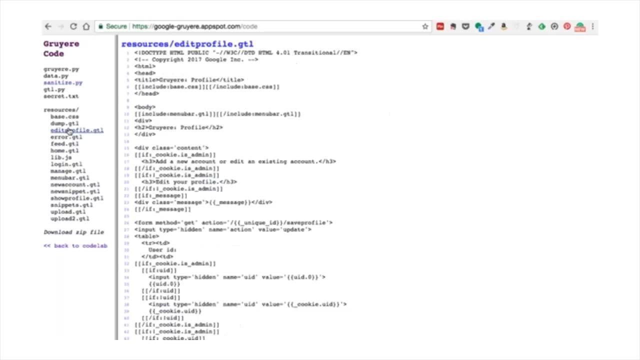 OK. so what if I try to see what the structure of this? hey look, I go to Code, I can see all the different files. and hey look, there's an Edit Profile and I can see all the code. 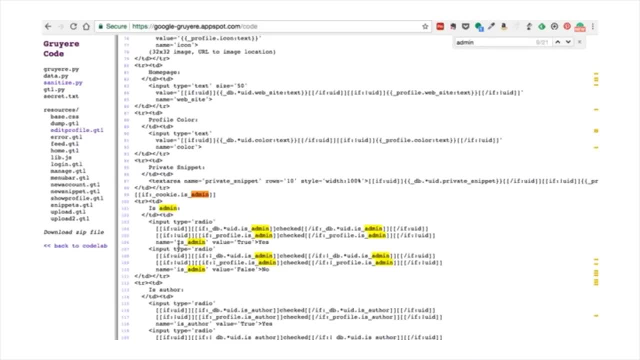 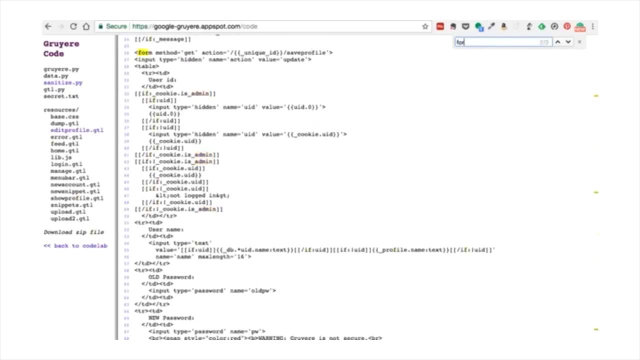 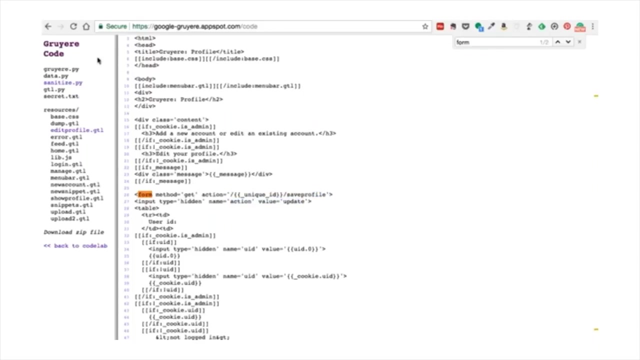 And now if I search for admin, I can see all these if statements that hide certain admin functionality from me. But now that I actually see how the file is structured and how everything is actually submitted through the form, and that we're submitting it through Save Profile with the 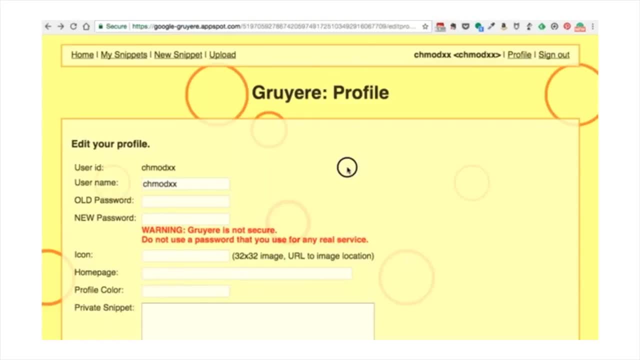 update value. I can actually go and just make myself an admin. So, instead of Edit Profile, I'm going to save the profile. Use the Edit Profile, Use that request and I'm going to pass my action as update and I'm also going to pass. 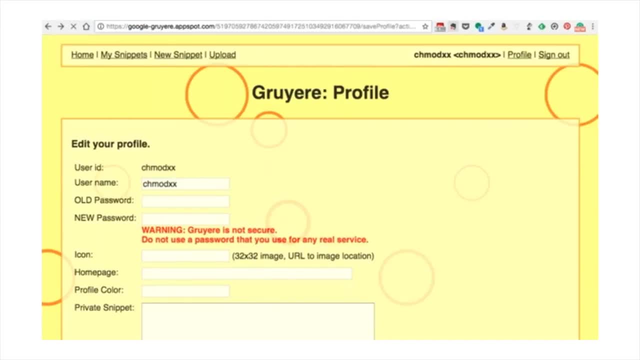 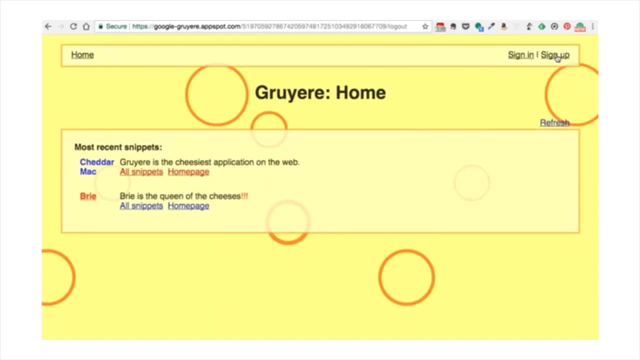 the is admin variable and I'm going to set it to true parameter. sorry, set the parameter to true. Now, if I sign out and then I sign back in, put in my username and password just as I did before. all of a sudden I have this new fancy button that lets me manage the server. 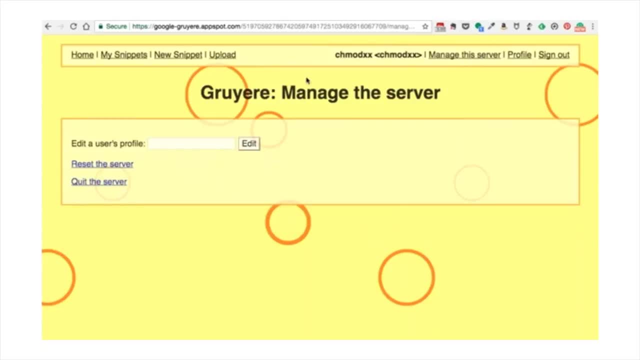 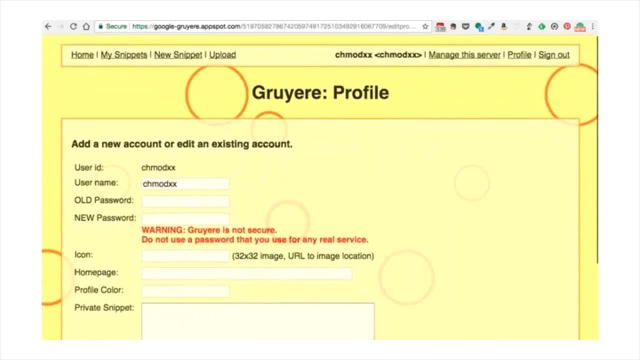 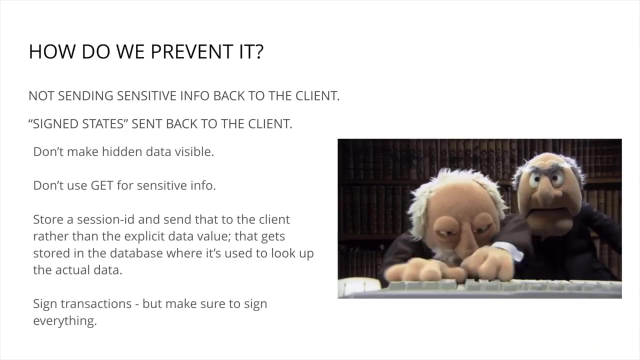 because suddenly I'm an administrator And I can reset the server, I can quit the server, I can edit any user's profile, and I did not have permission to do that. So how do we prevent this- Told you, I'd say it a bunch of times- but not sending sensitive information back to. 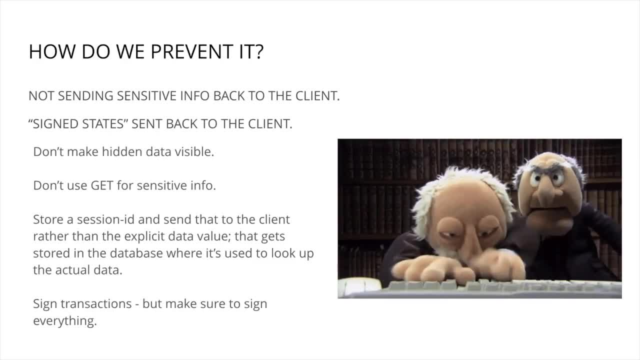 the client is rule number one. If you're going to send information back to the client that is sensitive in nature, make sure you're sending it in some sort of signed state. You also don't want to make hidden data visible And you don't want to use get for sensitive information because that can be manipulated. 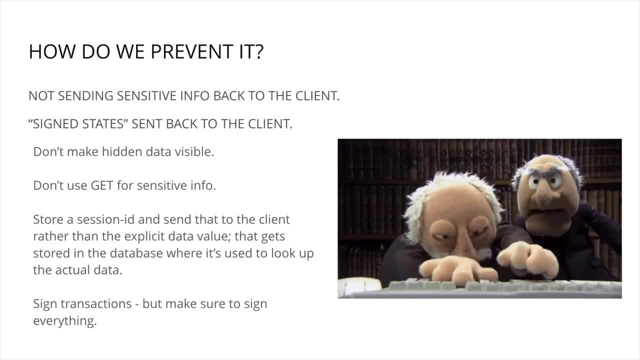 super easily. Post requests can also be manipulated really easily And you know you can. You can, You can stop the request midway and look at what information is actually being sent, And so just don't assume that just because you're using a post request, that you're actually 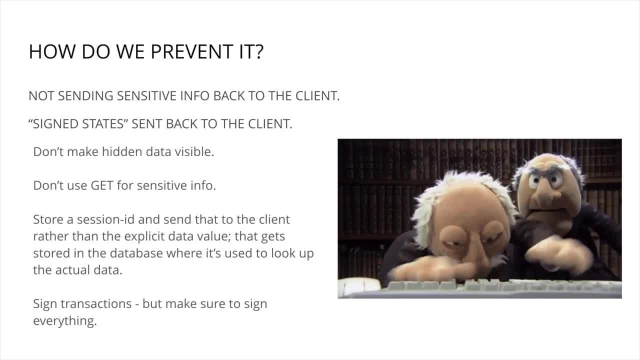 more secure. Just make sure that your state is signed, Or use something like a session ID that sends that to the client rather than the explicit data value. So, for example, something like the $7.60 for a large pizza wouldn't actually be returned. 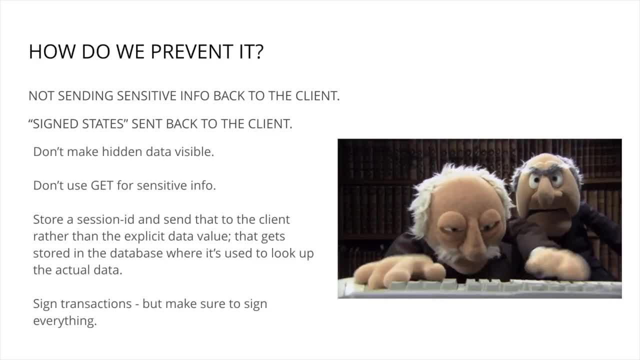 to the client as $7.60.. It might be some long, valuable deal. It might be a double-de-goop string of characters or numbers And then that is stored in the database and used to look up what the actual value is for. 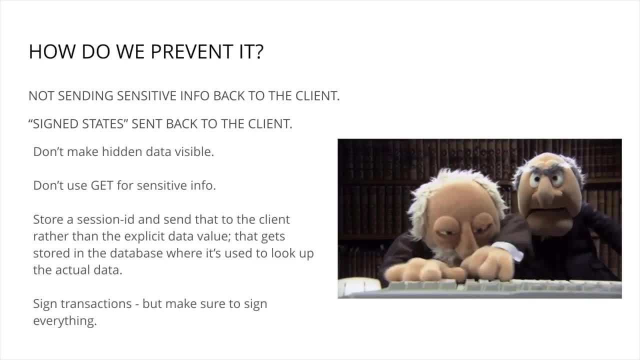 that price If you don't sign everything. a signature can be generated by performing a legitimate transaction, So make sure that when you're talking about signed states, the entire, The entire transaction that you're sending back to the client is signed. An example of someone kind of getting around this whole signed state situation is: 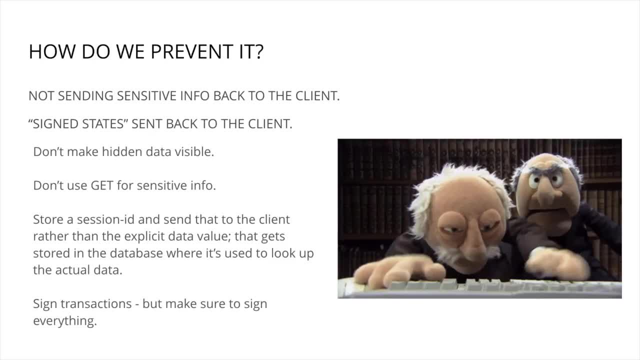 Let's say you only signed the price, So you've associated some sort of signature with a price and you send it to the client and you have to return the appropriate signature in order to make sure that the data that's being returned to you is legitimate. 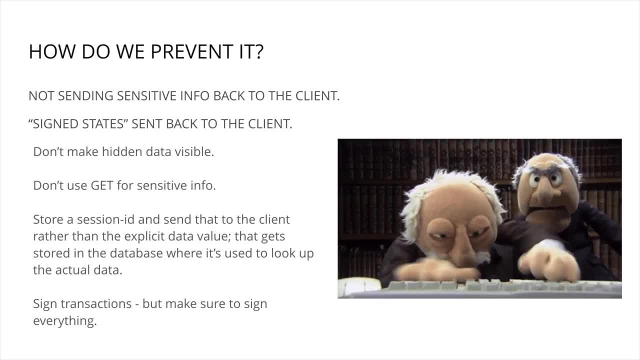 If you only signed the price, the attacker can actually go through the whole order process, get the signature for a super cheap item and use that to complete the purchase of a more expensive item Again. that would really only happen in situations where there's not very much security to begin. 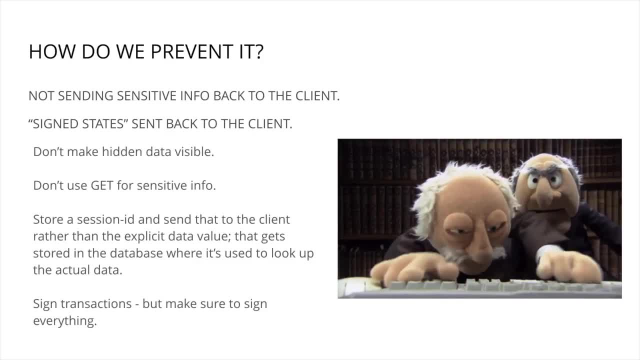 with, But to err on the side of caution and make sure that you are actually associating signatures for data with the entire transaction, so that someone can't say, Hey, I'm paying a $1.20 for this slice of pizza and I used the signature associated with. 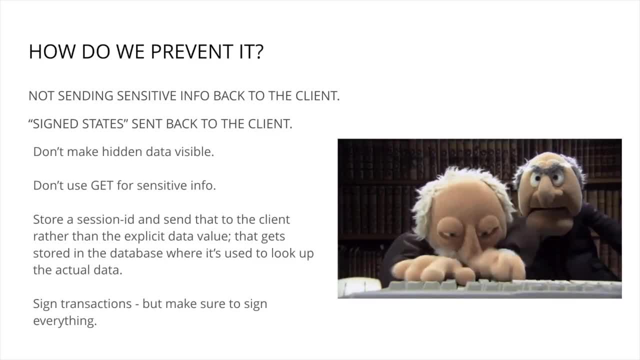 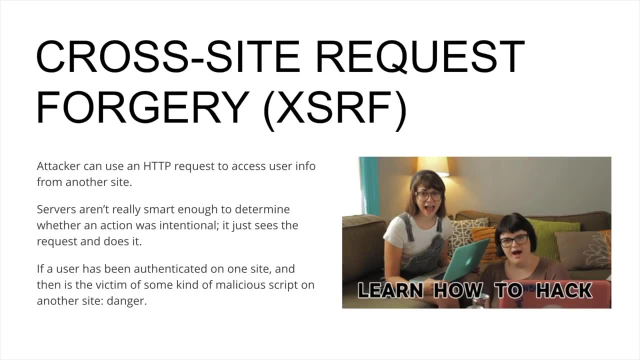 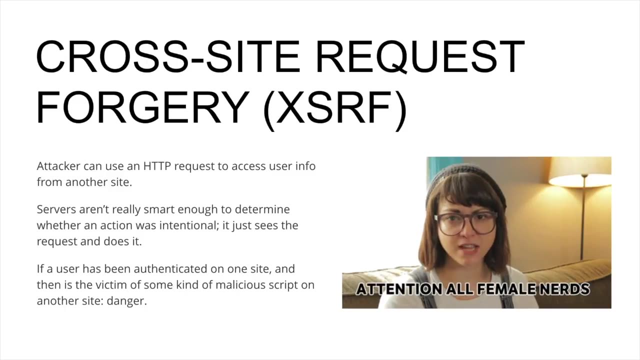 I don't know- Pizza Dip. That way, you can actually see that the large pizza was associated with the $7.60.. Cross-site request forgery: This is what an attacker can actually use: an HTTP request to access user information, your information, from another site. An example of this- and this example is used quite often: 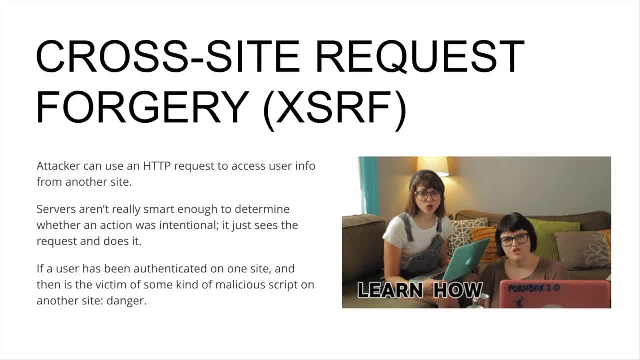 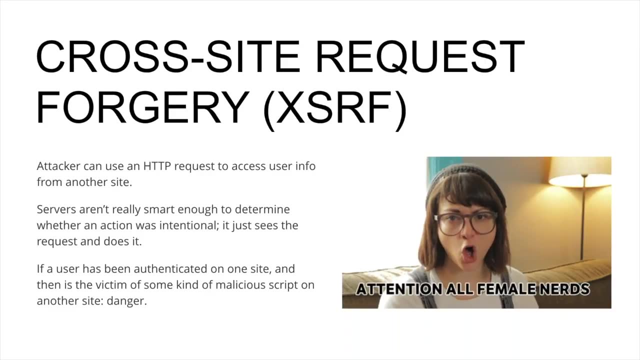 although it's not as likely nowadays. Let's suppose that you have a user who's logged into an online banking application And while they're logged into their bank, they also end up visiting some sort of sketchy website, And this website triggers some sort of attack that uses that. 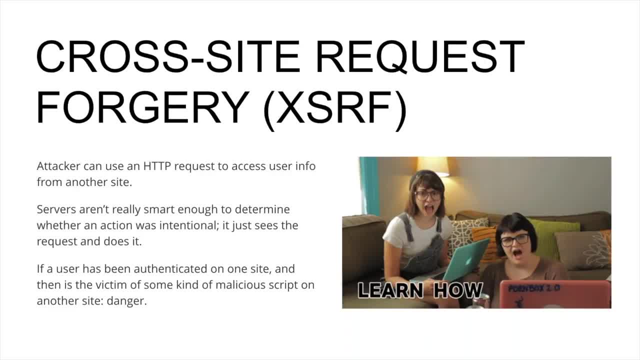 user's authentication to perform some kind of malicious activity, Let's say moving $1,000 from the victim's bank account to the attacker's. This isn't super likely because I would think that most of our banks now actually use tokens, as we'll see in the next couple of slides, And 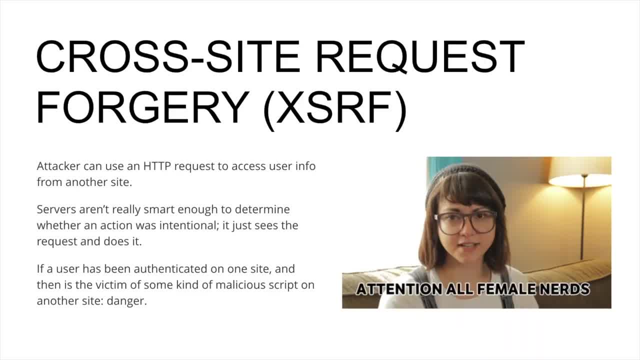 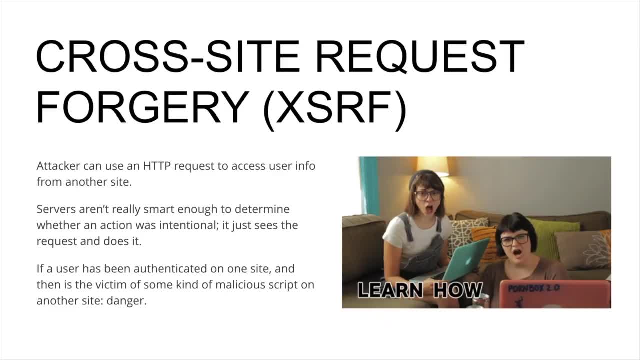 there is more authentication, because this would have happened to the bank already and it would have been disastrous, And so it's just not as likely that it would happen again because it would have been down that road, A more likely example of cross-site request forgery that I 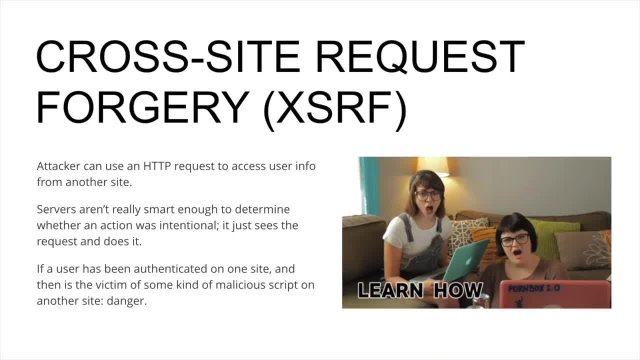 want to mention is something that could actually happen on a blogging site like Blogger or WordPress, And not that these are susceptible to cross-site request forgeries, but let's just use those as an example. So let's say that you're using some sort of blogging site that is susceptible, And 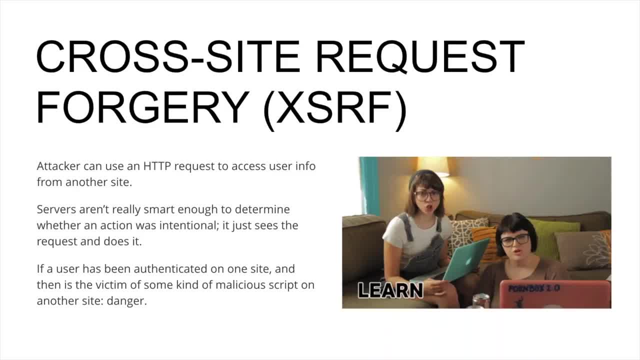 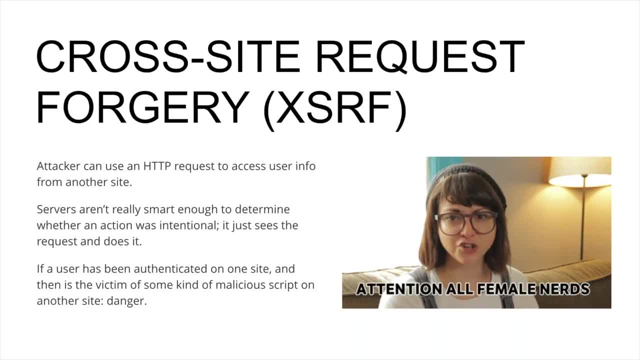 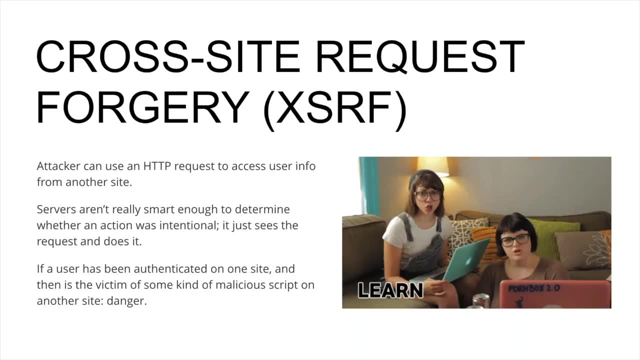 let's also assume the blogging app you use has some sort of request that takes the idea of the blog to delete. Like, let's say, you want to delete a blog and you pass that as a parameter to the request And that triggers a delete function. So some attacker on their own blog could actually 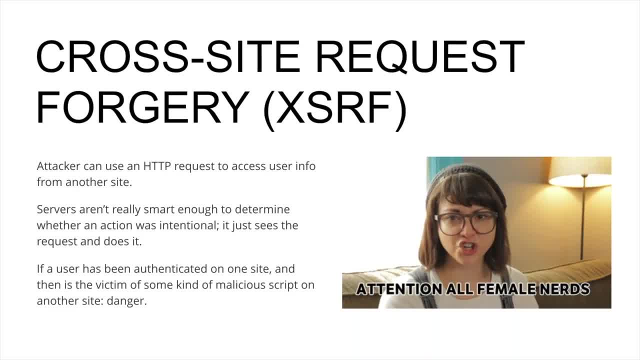 replace legitimate links on their blog with a request calling for the application to delete the blog of whoever's logged in and visiting the attacker's site. That is something that could very easily occur, And it's not necessarily something people often think about, but a lot. 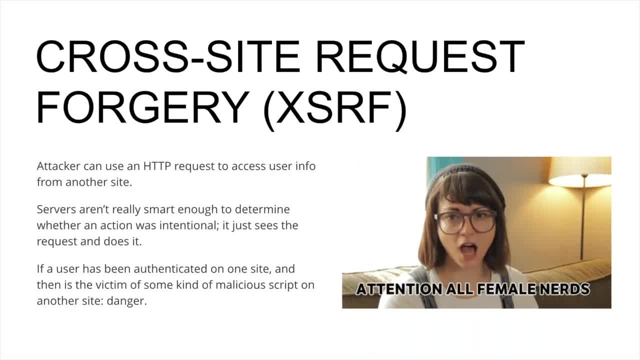 of blogging applications do give you the ability to, within your template, say, get the current user's ID or the current user's blog ID. So that is a possibility if cross-site request forgery is not being applied, And so that's something that could very easily occur And it's not necessarily. 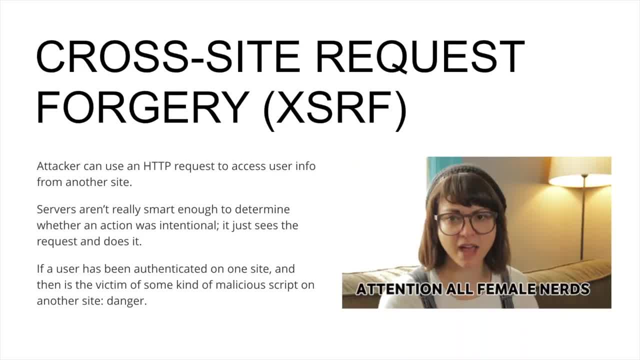 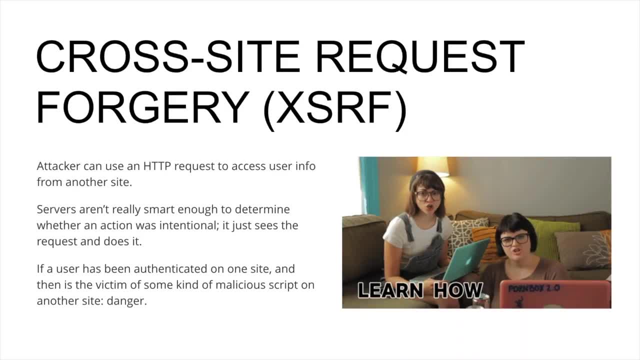 something that could be done by a blogger. So we know that servers really aren't particularly smart. They're not really smart enough to determine whether an action was intentional or whether it was sent by some sketchy person on a different website. It really just sees the request and it. 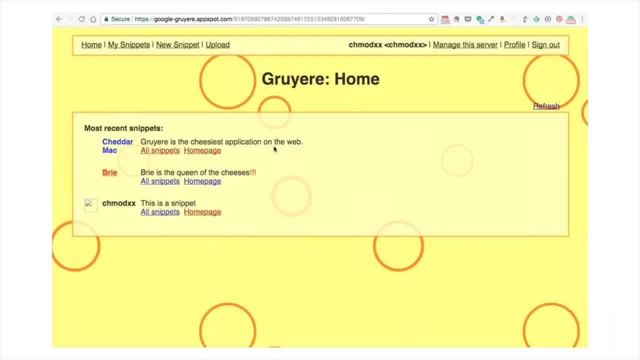 performs it, And we're going to see an example of that right now, And this basically follows the example of the blogging app that I mentioned on the previous slide. So here I'm seeing what request is needed to trigger the delete snippet function, So I'm going to. 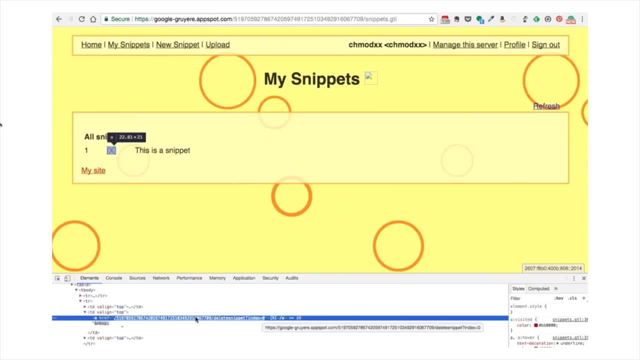 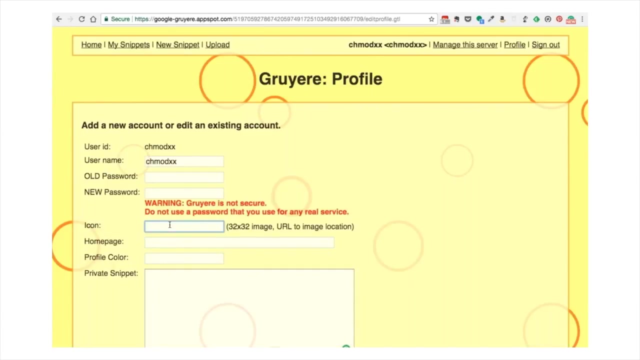 look at this. I see delete snippet and then I pass an index value. Okay, So I'm going to copy that. Now I'm going to go to my profile And I'm actually going to use that request URL as a little decoy for. 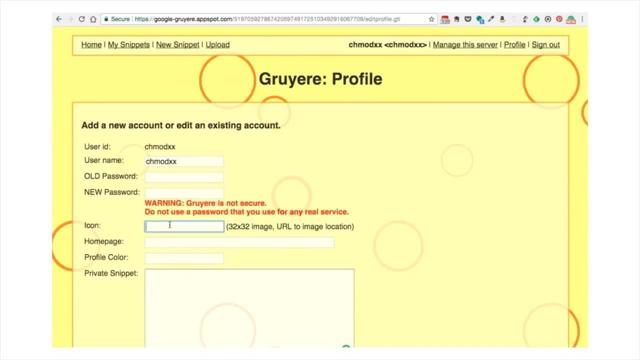 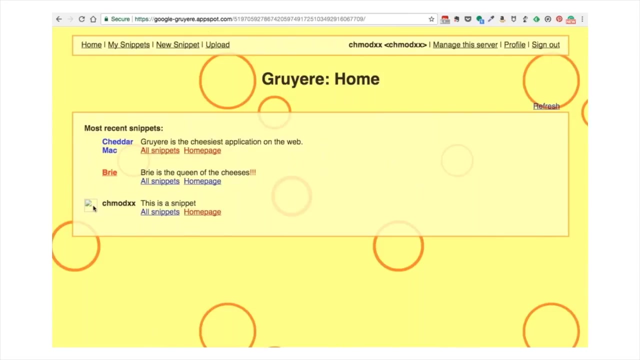 my profile icon. So whenever that icon loads, the server looks at the URL of the image at that delete request. but there is no image. But because it's looking for the image at that delete request, it's going to see that request is still actually calling the URL. So there we go. There it is Now. if I go to my 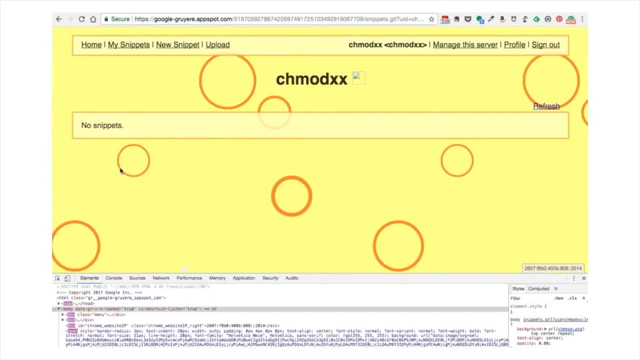 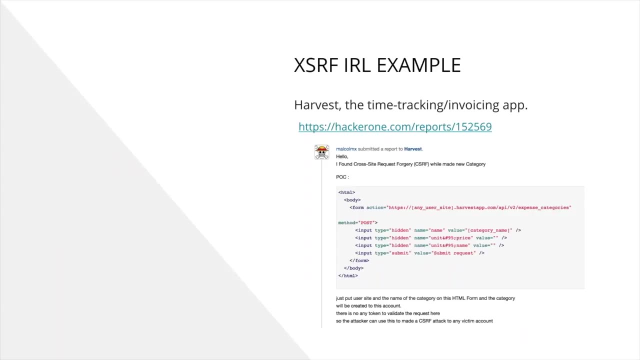 snippets. I did have one before and suddenly they're all gone. So here's an example of a cross-site request forgery in real life, And this is from Harvest, the time tracking and invoicing app. They didn't have token validation for creating a category for the request, So I'm going to go ahead and 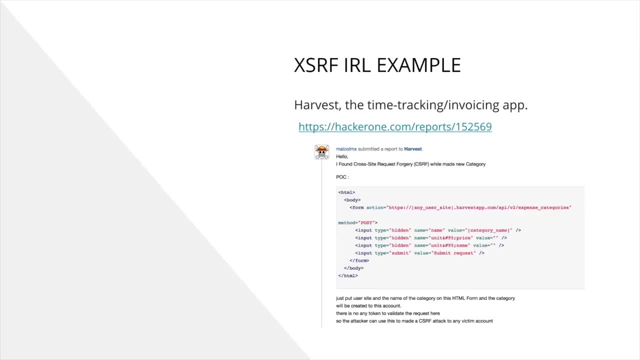 create a category for any user. So if you already had a Harvest account, you could actually just create a category for any other user site, any other company that happened to be using this Harvest application, and name it to whatever you wanted. And again there's the HackerOne report. if you'd. 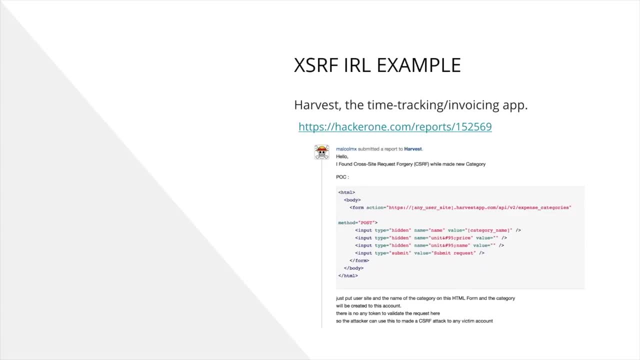 like to take a look at it. This is a less severe report than the cross-site scripting attack that we saw with Uber. So, as a result, this ethical hacker was paid something like $100 because Harvest did consider this a huge issue, But it is an example of a cross-site request forgery attack. So how do we? 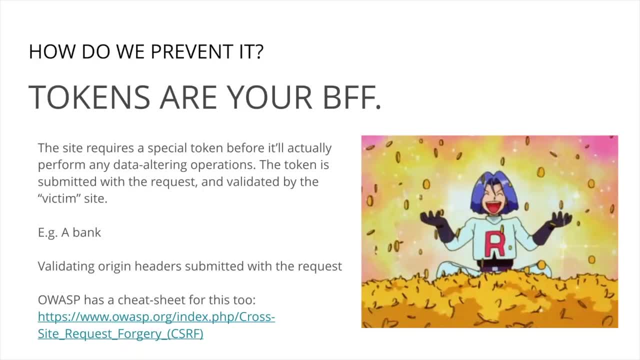 prevent this: Tokens. Tokens are your best friend And this is what banks use. Banks really use this tokenization to authenticate a user, Because it's actually really hard to spoof some random series of numbers and characters. It's difficult to do So. the site requires a special token before it actually 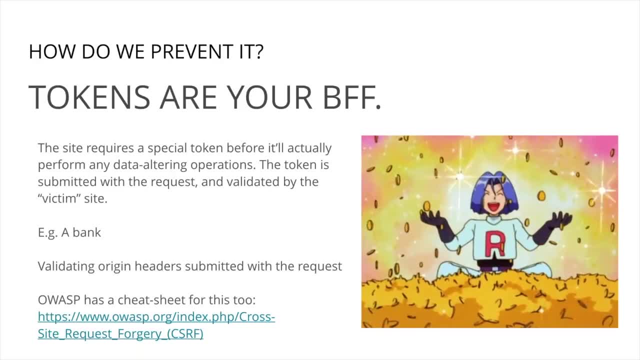 gets to the victim So you can use it to authenticate, and then it's submitted with the request and validated by the victim site. The other thing you can do is validate origin headers submitted with the request, And OWASP has another cheat sheet for this that I suggest you check out, just like the. 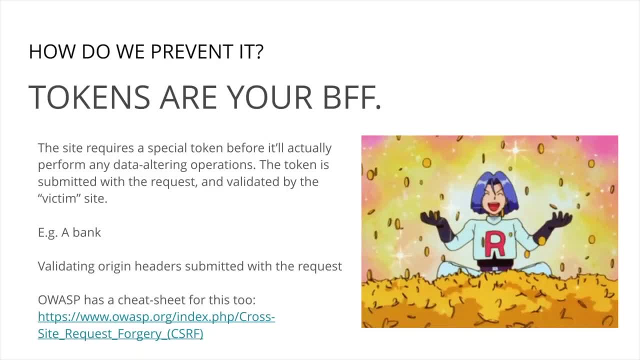 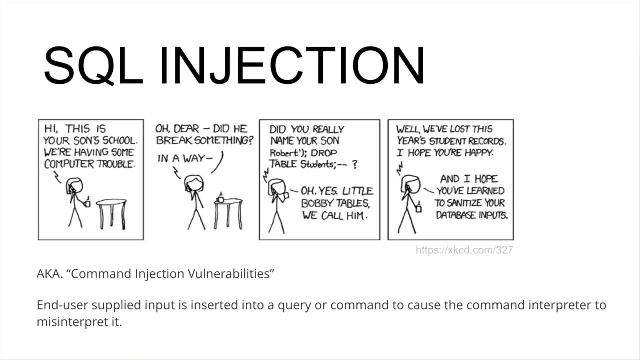 cross-site scripting cheat sheet, And they have a great example of how to basically run through all of the different preventative measures. Finally, we're going to talk about SQL injection, So I figure any of you who read XKCD have probably heard that word before, And so if you're learning to do it, you might be able to do it at home, And then you can also download it on your computer, And you can do it at your computer. If you're not familiar with it, you can download it on your computer, And this is a very, very 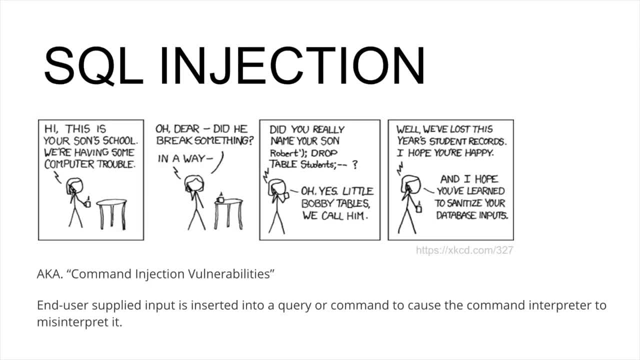 seen this comic strip and it's pretty great. it's a really good example of SQL injection. Another name for SQL injection is command injection vulnerabilities. So the end user supplied input is inserted into a query or a command that causes the command interpreter to misinterpret it. So we're gonna see an example of this. 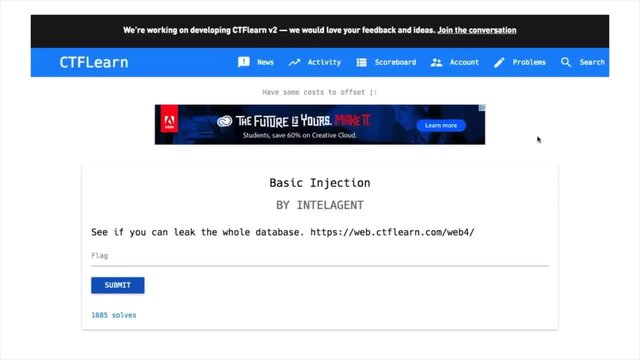 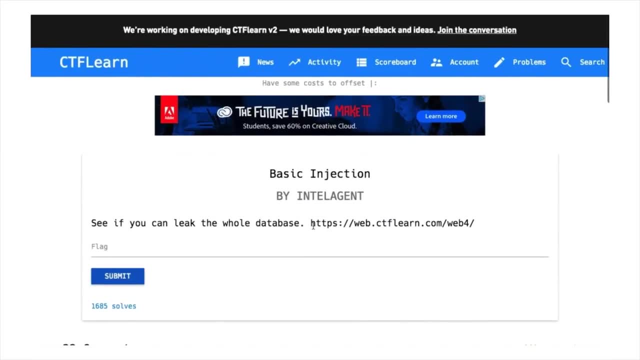 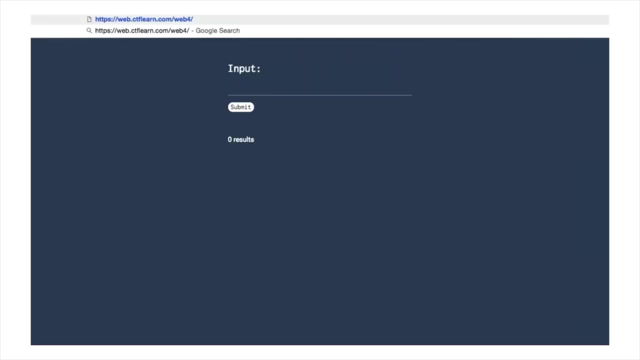 right now. So I can tell this is some kind of form and this is actually on a CTF learning application that I'll talk about in a little bit. So I see this input, I know it's some sort of form. I don't exactly know what it does, so I'm. 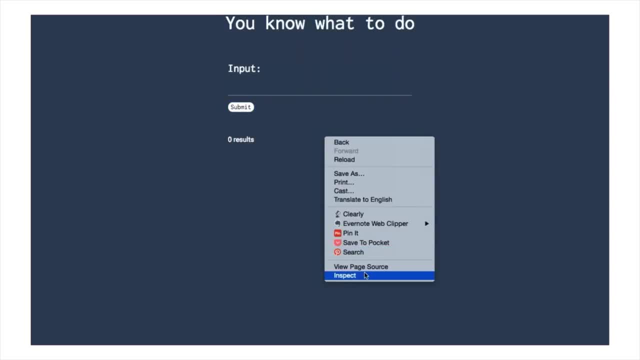 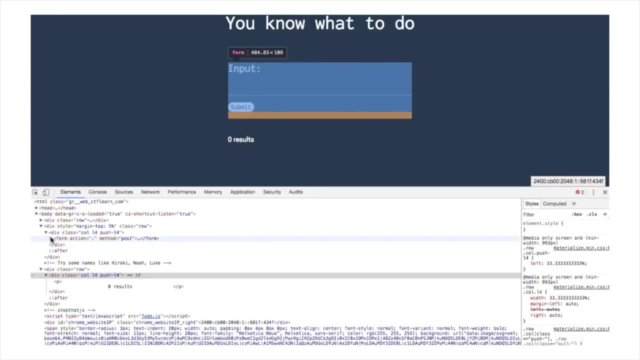 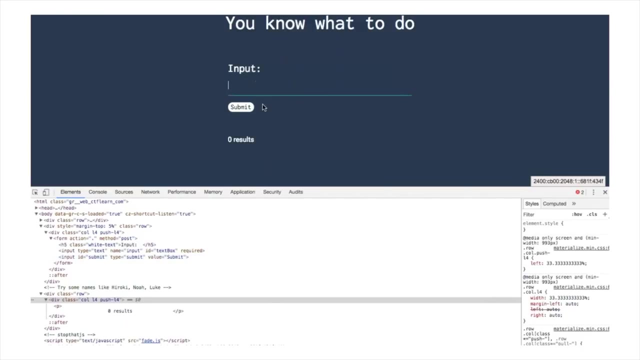 just gonna throw in some dummy text hoping it'll tell me something. It doesn't really show me anything, But I can see that it submits something somewhere. There's a submit button, there's the form action. So I must go somewhere. it's a form, So I'm going to. 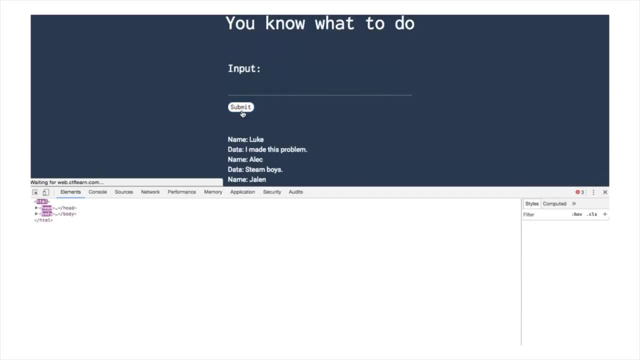 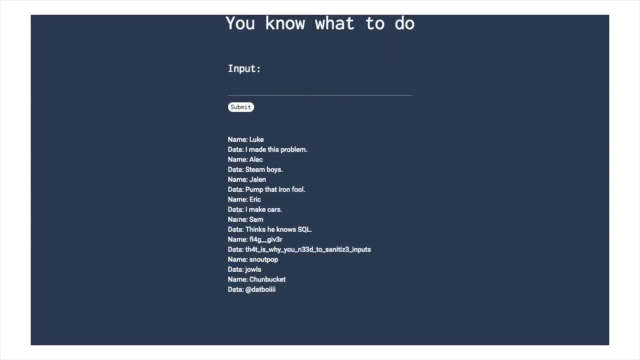 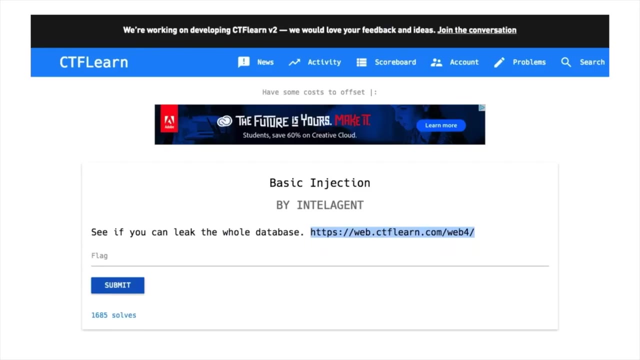 throw in this potentially malicious breaking SQL query. There we go. So what happened is I actually broke the database query. Broke is sort of an inaccurate description, But I essentially finished off the query saying: you know, one always equals one, So that's always gonna result true and, as a result, the database actually 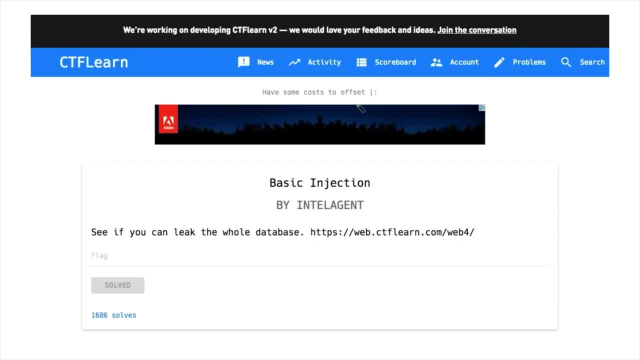 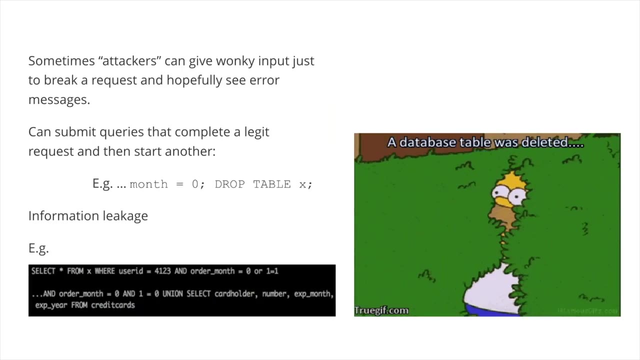 threw back all of the all of the data that it contained, and I was able to actually access all of that data. So that just means that their SQL queries weren't being sanitized. Sometimes attackers can give wonky input, So that's what I-. 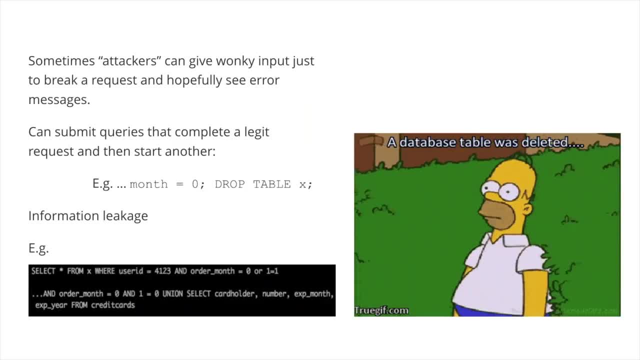 breaking. You know there's a couple ways that you can quote, unquote, break a query. One is to really just, you know, give an input, give weird input that just totally breaks the request, and hopefully see some error messages that pop up on the screen So you can kind of get an idea of how the 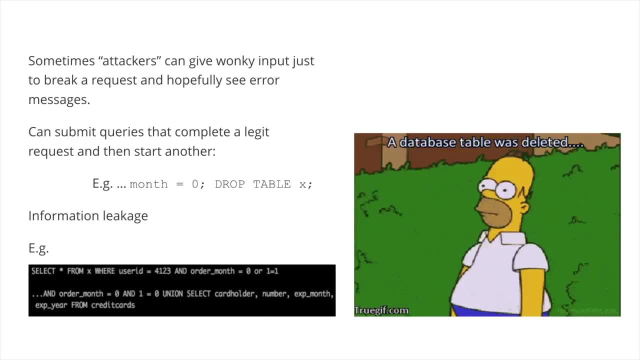 application is configured And then you can also submit queries that complete a legitimate request, as we just saw with the one equals one, Or for example, here month equals zero, and you finish off that query and then you can say: drop table X. And here, if you do this because there is 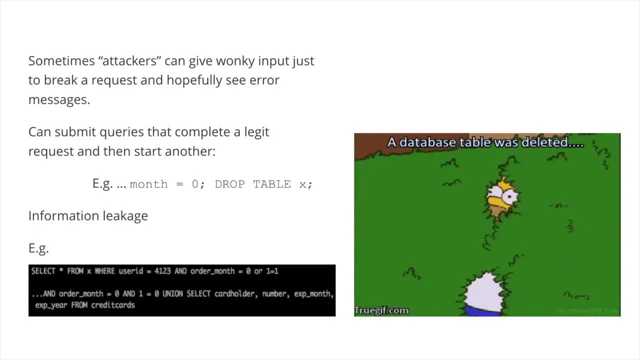 presumably no month zero. the first half of that query, whatever it was supposed to do, doesn't actually do anything, So that finishes. It says okay, well, I have nothing to do, I have nothing to return Month, there's no zero month. So let's go on to the next instruction, dropping table X. 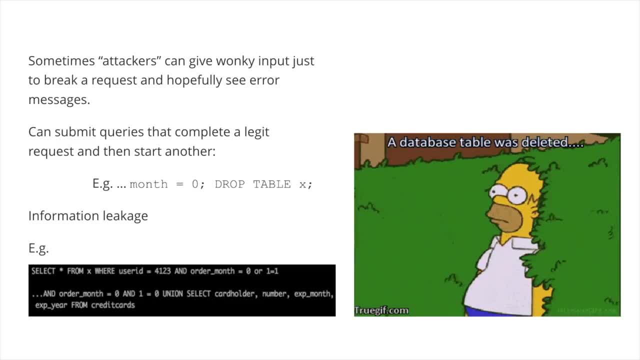 That is dangerous, because now you've just lost an entire database table. It can also result in information leakage, as we just saw in that last demo. So here's an example of that: Selecting star from X, where user ID equals this and order month equals. 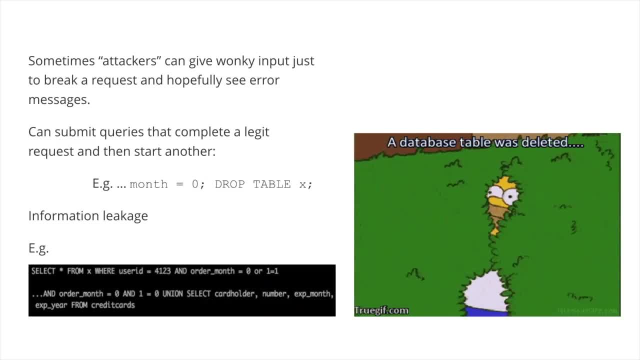 zero or one equals one. One equals one will always be true. So that will be evaluated And you can say the order month equals zero and one equals zero. And then you can select all of the card holders numbers, expiration months, expiration years from credit cards And that will actually 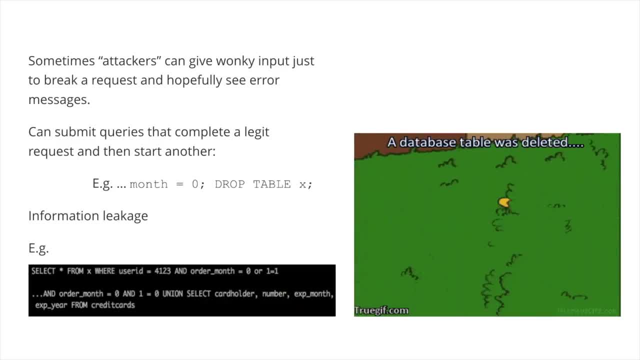 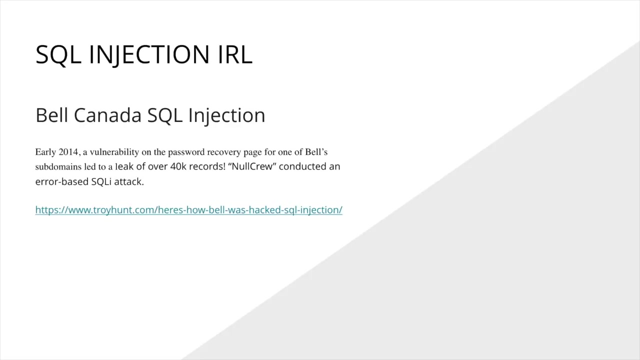 be joined with the lack of data you received from the previous query, So you won't actually get any customer orders in that result. But because they specified that union, the database will still retrieve the information from the credit cards table. Here's an example of SQL injection in real life And this actually happened in 2014.. Bell Canada. 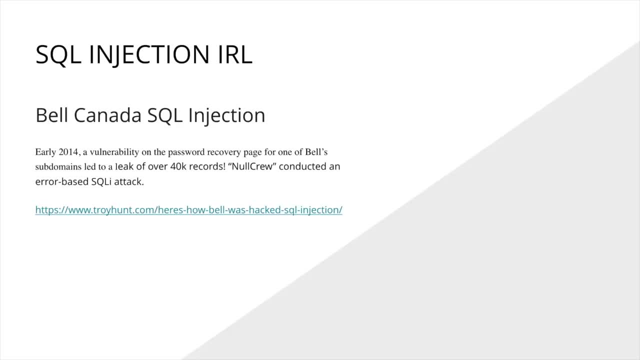 a big company here in Canada, was attacked by a hacking collective called Null Crew, And they used an error-based SQL SQLI injection attack. So this actually ended up in basically leaking over 40,000 records from one of Bell's subdomains. It was all through a vulnerability in their password recovery page. 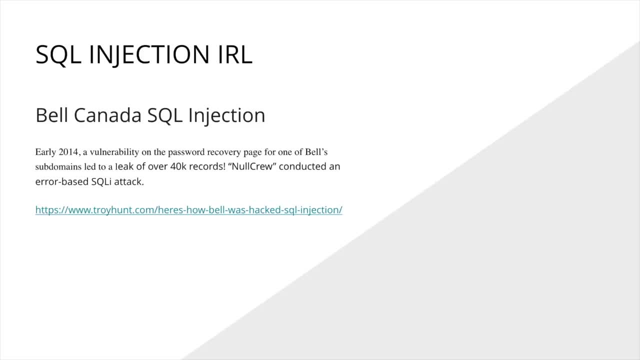 And Troy Hunt. if you've heard of him, he's basically a security legend. He's responsible for the super helpful site Have I Been Pwned, which tells you when you enter your email address, you can see whether that email has been involved in any sort of security breach. His blog is also. 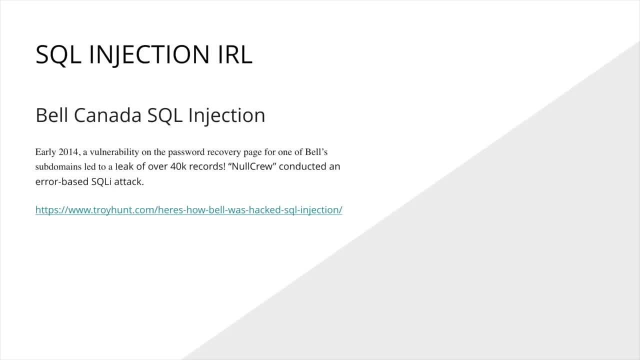 full of tutorials and explanations and reports. It's a really great learning resource. And he actually steps through this entire attack and recreates it with his own ASP password recovery page. So I really suggest you check that out if you have any interest in this particular attack. 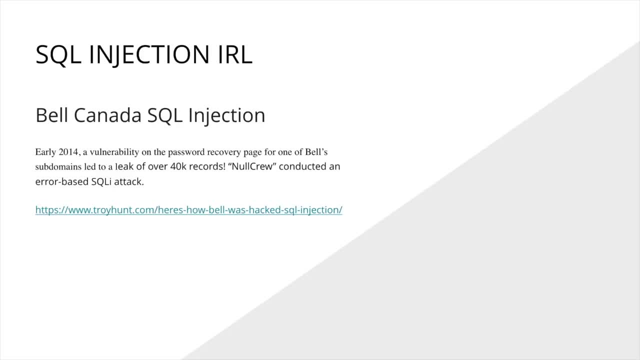 factor. It was terrifying and interesting at the same time. So how do you prevent SQL injection attacks? So how do you prevent SQL injection attacks? So how do you prevent SQL injection attacks? You have to have multiple attacks per second, And this is something that has to be. done in two different ways. So, for example, you can find multiple attacks in 24 minutes. You can find multiple attack vectors in six seconds. You can find multiple attack vectors in three blocks per second. If you find multiple attack vectors in six seconds, it's going to change the 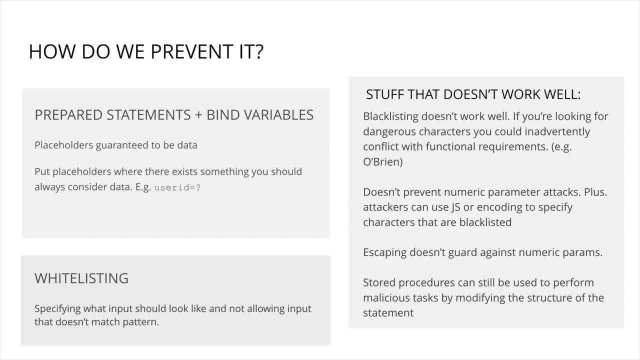 and bind variables. So these placeholders are guaranteed to be data And I'm sure a lot of you have seen them if you've worked in certain frameworks like Laravel with PHP has them. So you put placeholders where you're going to actually put or submit something that should. 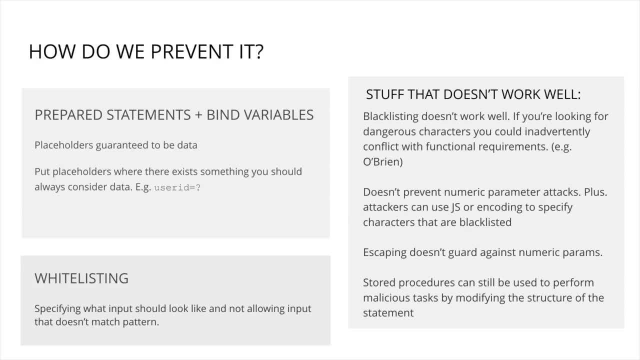 always be considered data. So for example we see here user ID equals question mark, So that question mark will always be data. It cannot be essentially run as some sort of query And you don't have to worry about it being past the database, Even if someone passed in something. 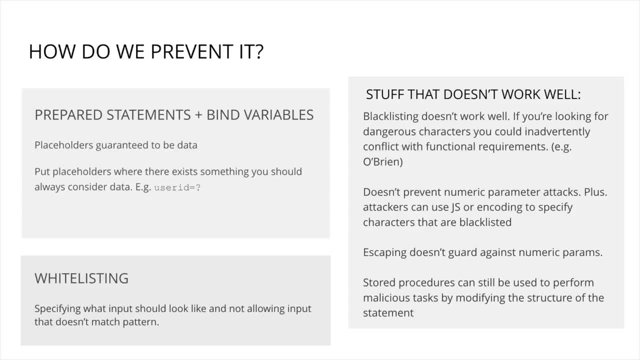 like one equals one semicolon, drop table X. that would still just be seen as data And presumably your database would be set up so that it could only take integers for the user ID And it would just throw out an error saying, hey, that's not an integer- Whitelisting- Whitelisting also works. 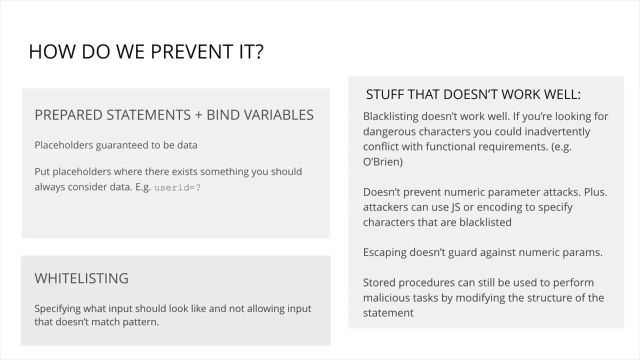 Specifying what the input should look like and not allowing input. that doesn't match a pattern And that's kind of similar to the prepared statement And it essentially again just tries to make sure that whatever is being passed to the application is what it says it is. So you set up some sort of pattern that really 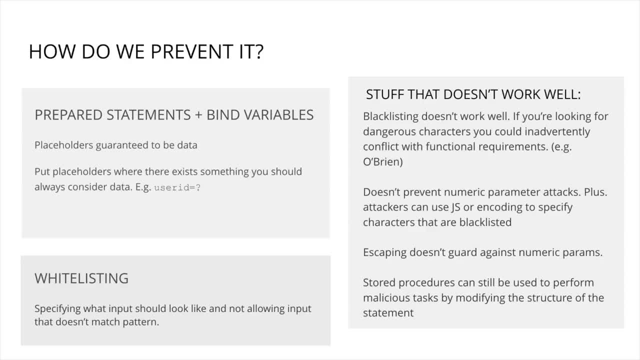 wouldn't match some sort of SQL query. It has to be data, It has to be an integer or a float or a string or whatever else. Some things that don't work well, that some people have implemented and it's really not particularly secure. Blacklisting doesn't work particularly well. 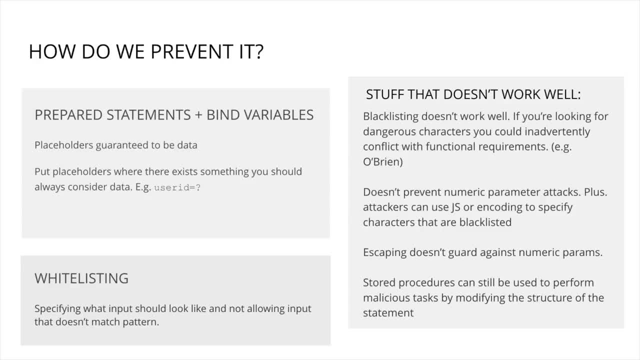 So if you're looking for dangerous characters, like a single quote mark, that could conflict with functional requirements- So, for example, my landlord's name is O'Brien And if you were blacklisting that single quote, then all of a sudden he cannot be entered in a database anywhere. 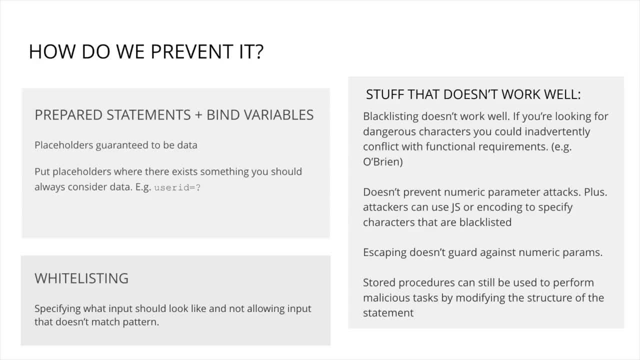 Blacklisting also doesn't actually prevent numeric parameter attacks, And attackers can really just use JavaScript or some sort of encoding to specify characters That are blacklisted, And you basically have to go through all of the different possible encodings to blacklist those And it's just kind of messy. So it's just better to err on the set of caution. 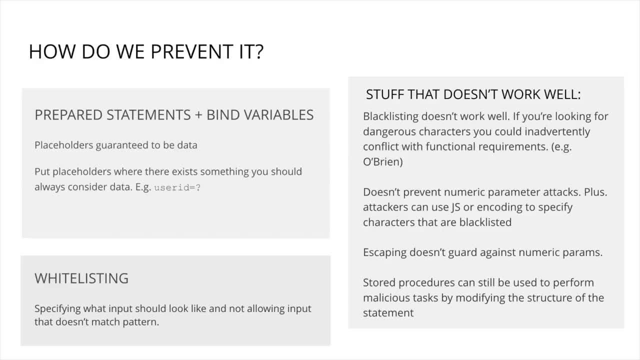 and not rely on blacklisting. in that way, Escaping doesn't actually guard against numeric parameters, So that's really not the best approach either. And then sometimes people talk about stored procedures, And those can actually still be performed to use malicious, or they can. 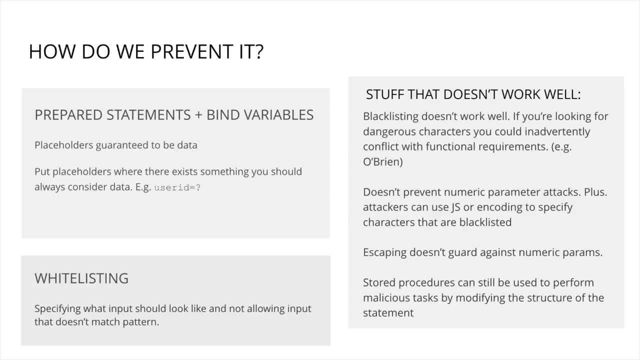 be used to perform malicious attacks because you can just modify the structure of the statement. So really it's best to stick with prepared statements and find variables and white listing and kind of avoid the stuff that could work but still has the potential for vulnerability. 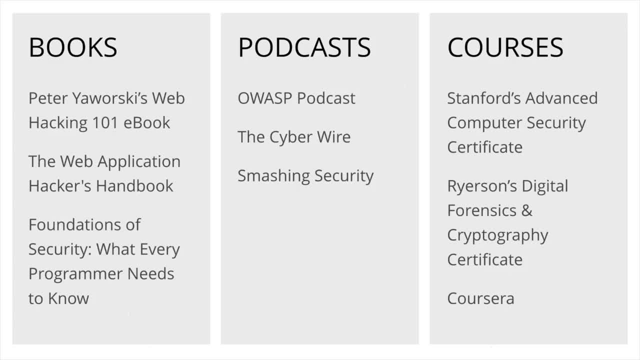 So now we're going to talk about how to keep learning. There are some incredible books for web application security and web hacking. I really suggest you check out the Web Hacking 101 eBook. It's written by my coworker, Peter, who literally wrote the book on web hacking, And the foreword for this book was written by the guys. 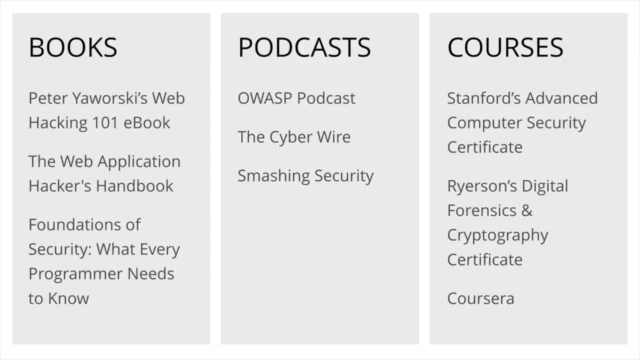 who founded HackerOne, which is our Bug Bounty program as well, And it's just an invaluable resource. It is an application developer And it's available online And it's really affordable, So I would definitely recommend that. one Another great book is the Web Application Hacker's Handbook. 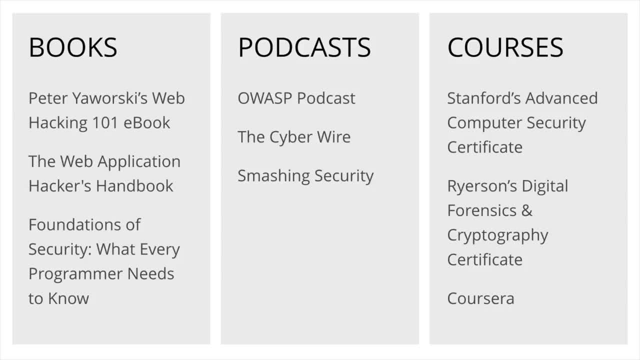 This is another excellent resource. It's been used from certain courses that I've seen as kind of like the textbook for students. And then, finally, Foundations of Security, What Every Programmer Needs to Know. This textbook was written by the professors who teach the security foundations. 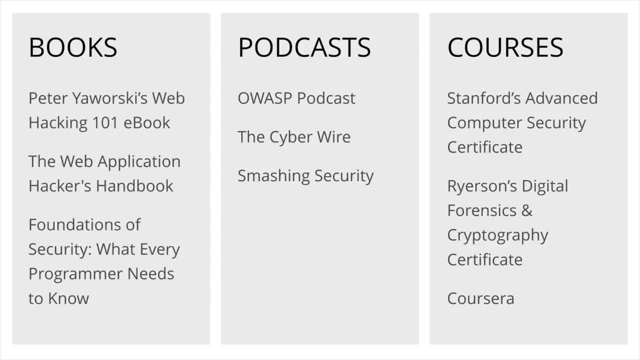 course for Stanford's Advanced Computer Security Certificate And it's also a great resource. It's very easy to see and it's really helpful And it's really helpful for those who are looking for a job. It's really easy to see how the attack vectors they discuss can be applied to everyday. 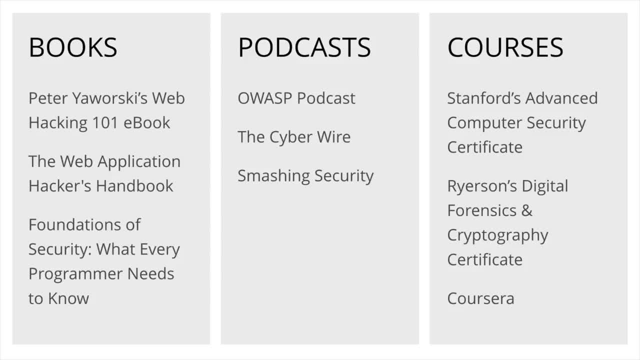 web application development And it's really user-friendly- Podcasts. So OWASP has actually put out a podcast. So I suggest you take a look at that, because they talk about a whole bunch of different issues, not just tutorials and stuff, but also recent attacks and kind of like cybersecurity. 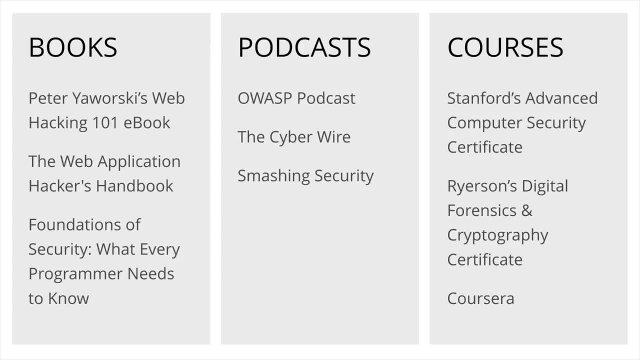 in the news, And then, finally, Smashing Security. I listen to Smashing Security every single week. It is less about how to avoid certain vulnerabilities, and not necessarily specific to web security, but they do talk about any major breach that has popped up in the news And the 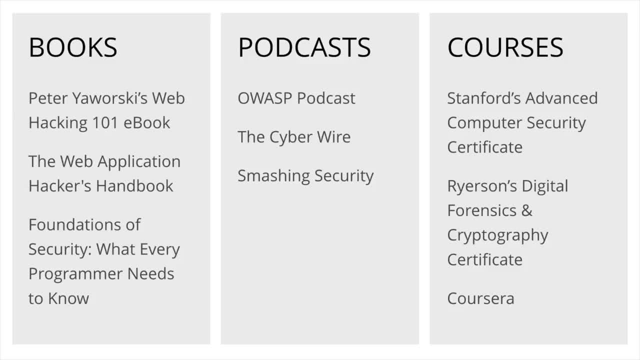 two hosts have been in the industry for years and years and years and they just have a great rapport with each other. I burst out laughing on the bus listening to them. They're really great. And then, finally, Courses. So I'm really only talking about these courses because I have experience with them. 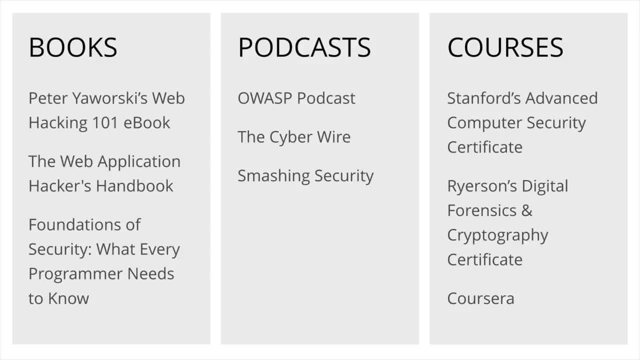 I've enrolled in Stanford's Advanced Computer Security Certificate and it's great for anyone who doesn't necessarily want to go back to school in person and take a course in real life with a professor. All of their lectures are recorded online and readily available. Again, the 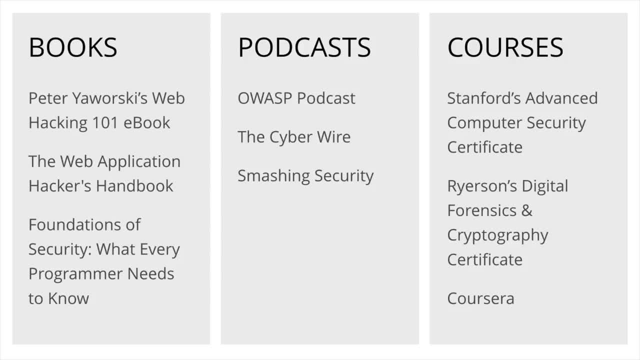 professors for this wrote the Foundations of Security book and they cover everything from Security Foundation and then they cover all of their courses. So I'm really only talking about these courses because I have experience with them. I've enrolled in the Stanford's Advanced Computer. 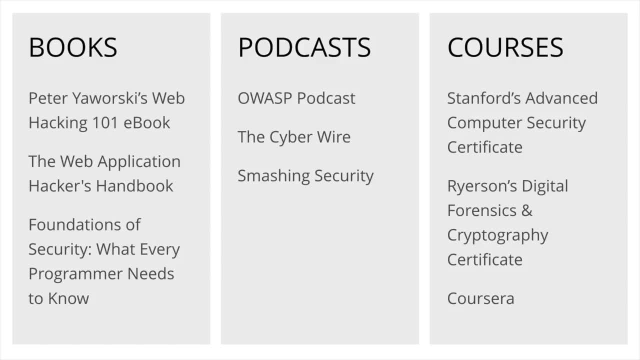 Security Certificate and they cover everything from Foundations to Web Security, to Mobile Security, to Network Security. There's kind of everything you could possibly need in that particular certificate program. For anybody in Canada who knows of Ryerson University, or in the States, they also offer an online-only option for their security certificate program, And I'm also in this. 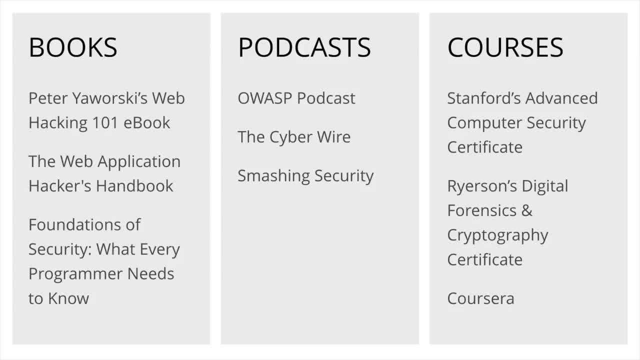 I'm also a student in this particular program and it's great. The professors are actual computer science professors at the university and you submit labs and assignments and they actually review and give you feedback for a number of different courses. network security: 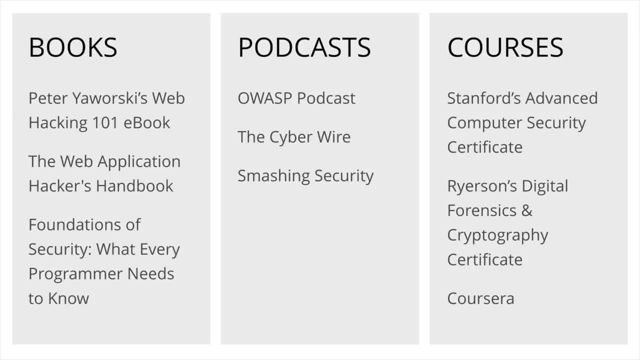 cryptography, digital forensics, mobile security. It's a really wonderful resource as well. And again, both of these are offered online. You don't actually have to be there in person, but they are not free, So there is tuition associated with each. They are about the same. 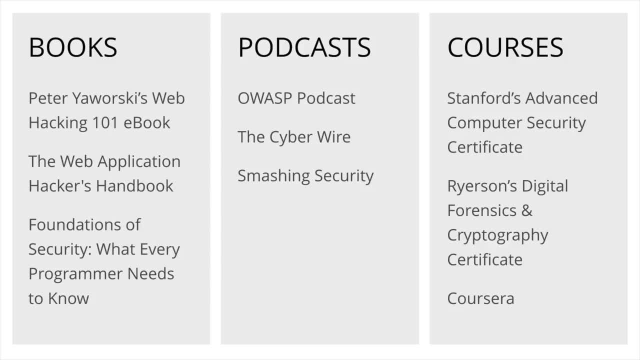 price when you factor in the Canadian and American exchange rate. but, as I said, they're not free. Coursera on the internet is also a great resource. It's a great tool to use when you're looking for information, but it's also a great tool to use when you're looking for information On the other. 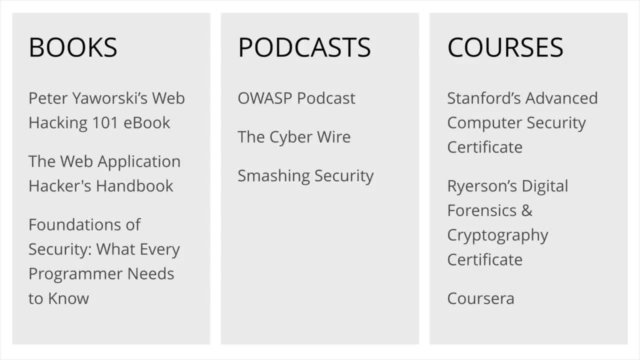 hand, it actually has a number of free courses available just right now- You could go after this webinar and look them up- And a lot of them are produced by actual security experts or professors and a whole range of different topics, So they are a great resource as well. 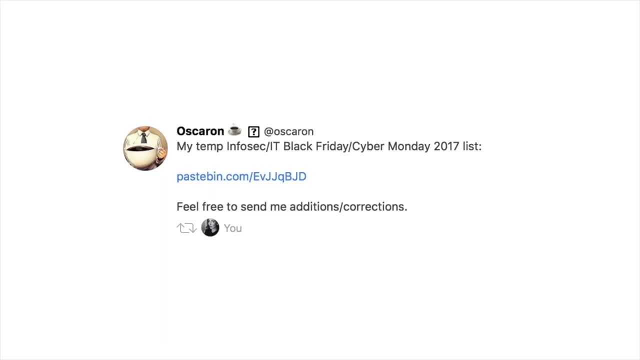 Now because we're getting up to Black Friday and Cyber Monday. for anyone who is interested in checking out some infosec software or books and stuff like that, this guy on Twitter came up with an entire list of all the deals coming up for this coming weekend. 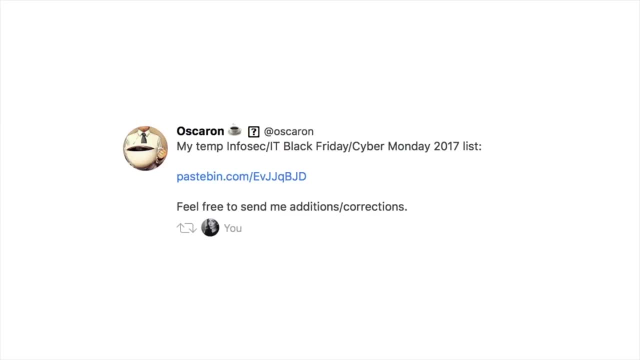 And again it's a pastebin. so I've taken a look at it. There's nothing sketchy going on there. He just happens to list all of these really great deals for certain software. I can't remember the name of the site right now, but it essentially lets you see all of 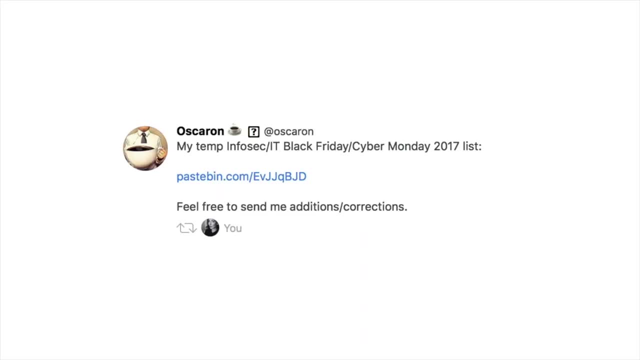 the Internet of Things devices that are currently connected to networks, And it's used a lot in IoT hacking classes. So if you're interested in that, their software is up there. And there are also some really great courses. There are some online programs, sort of like Udemy. 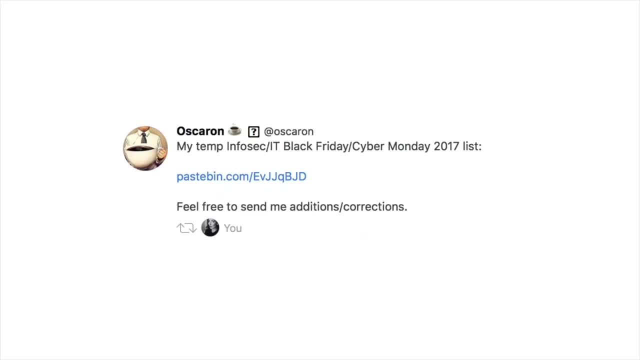 but specifically for security, And they're having a big sale right now. So instead of being like $100 a month to access their entire catalog, it's $30 a month. So if you're interested, take a look at that. There are some great educational resources there. 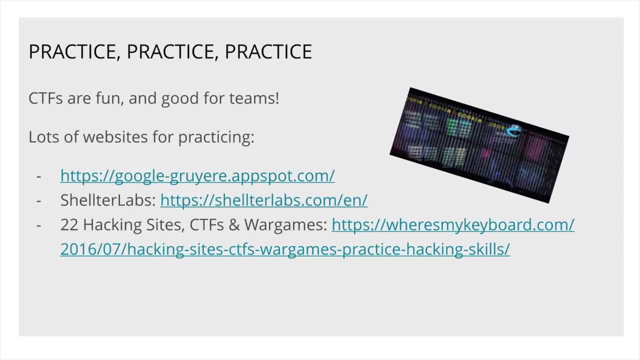 Now practicing, I think, is probably one of the most important things you can do, So we're going to take a look at some CTFs. For those of you who haven't heard of the CTF, it's short for capture the flag, And basically what happens is either by yourself or with the 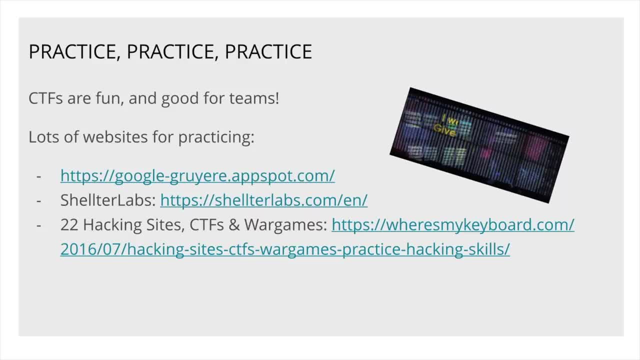 team. you are given vulnerable web applications or any kind of software and you have to look for certain flags. So, for example, it could be something like finding a cross-site scripting vulnerability in a web app, or it could be doing reverse engineering on a particular piece of. 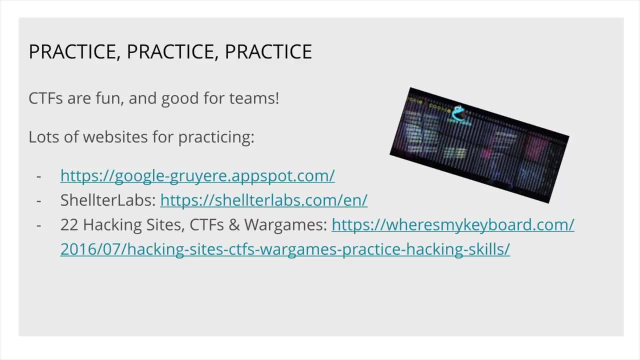 software that you've been given by the organizers And then you actually look through, you know whatever your particular assignment is and you try to find this little flag and they can be kind of structured in a number of different ways, But once you found that, you know that you found a vulnerability in that application. 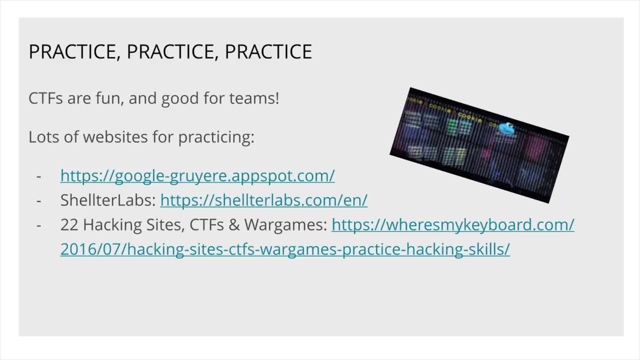 There are a lot of websites for practicing those where you saw those demos that I was doing earlier. That is actually an app that was developed by the security team at Google to help people learn about web security, And it is an amazing resource and a lot of fun to work through on your own as well. 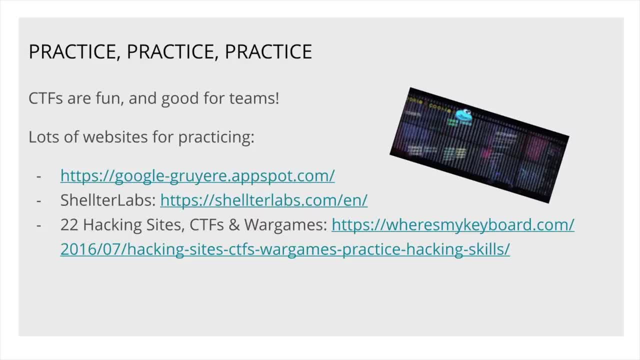 So that's a great place to practice. Shelter Labs is sort of like a social network style CTF. So you create an account, you can go through and find vulnerabilities on their site, And then there's this website as well, where there's a collection of 22 different hacking sites, CTFs and war games. 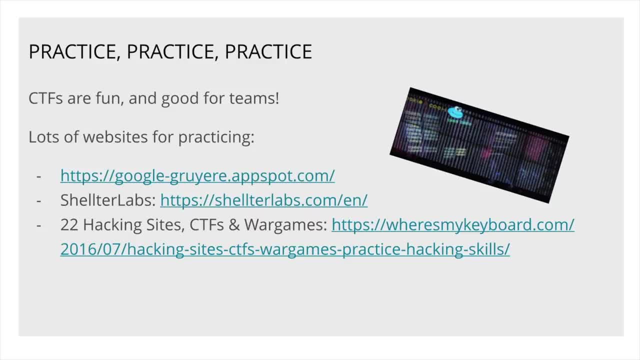 So, even if you don't necessarily live in an area where you can readily, you know, go participate in a CTF with a team or with your coworkers or with your friends or whatever, there are a lot of resources online And they're really really helpful.